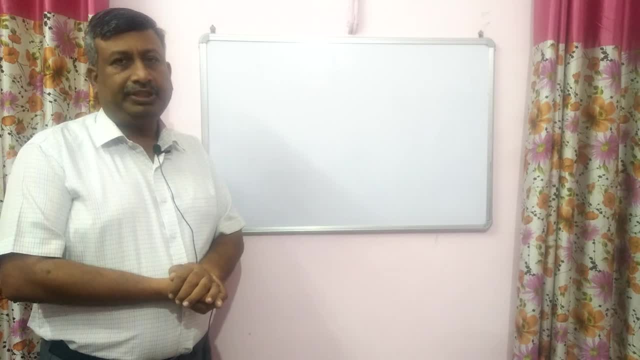 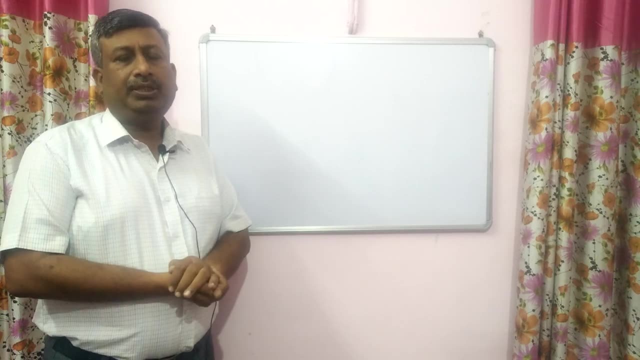 what are the impact of drought on plants and society? So drought is a condition. it is a dry condition when water quantity is not sufficient to fulfill the requirement. So this is a condition where water quantity is not sufficient So to fulfill the requirement. 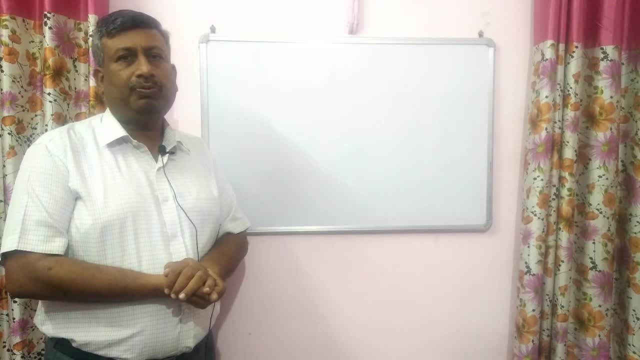 of plant or human being or any other requirement, water is not sufficient. That condition is called drought. So drought is a dry period, we can say, and it is different from aridity. There is a difference between aridity and drought. You can watch. 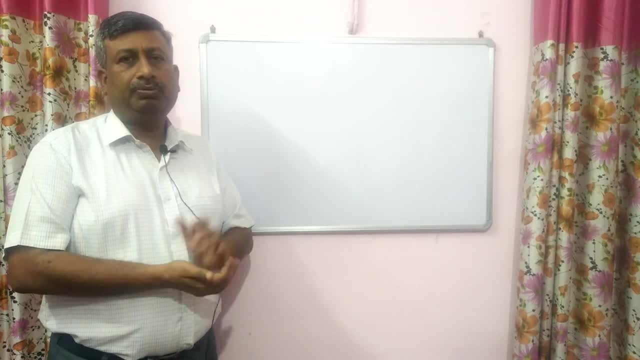 This lecture. it is already uploaded and you can go through playlist. Go to the RANFYD agriculture playlist. There are lectures on aridity and its importance. So from here you can see what is the difference between aridity and drought. Aridity is a degree of 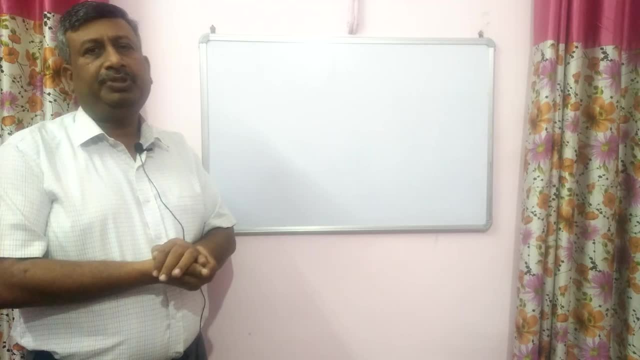 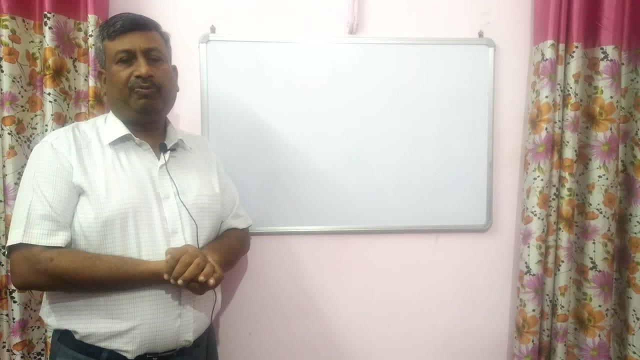 dryness which characterize the climate. So the objective of aridity is to characterize the climate. But drought is a dry condition when moisture in soil or reservoir is not sufficient to fulfill the requirement. So drought is a temporary in nature and it depends. 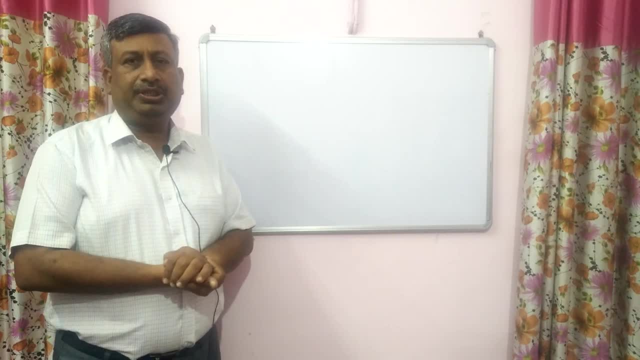 upon the rainfall characteristics, its quantity and its behavior. So this drought is very important. and in our country most of the agriculture is dry land. agriculture depends on rainfall condition, So drought is very common in arid and semi-arid condition. So 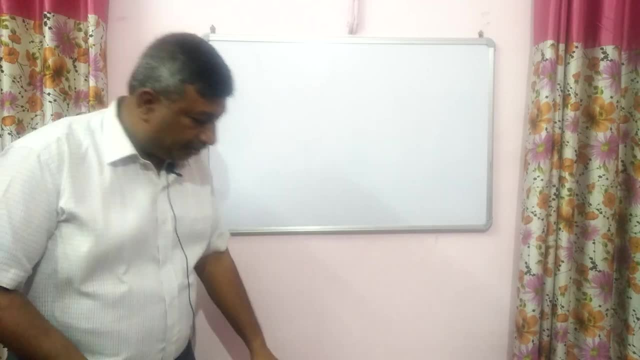 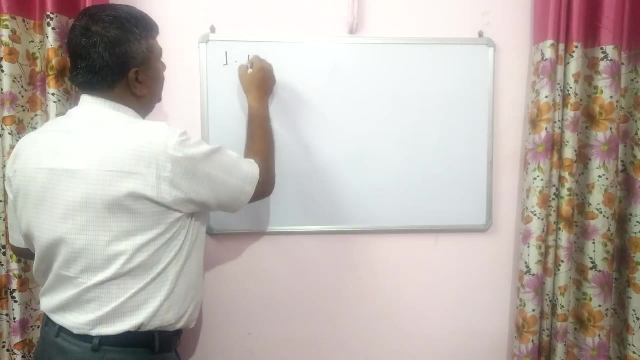 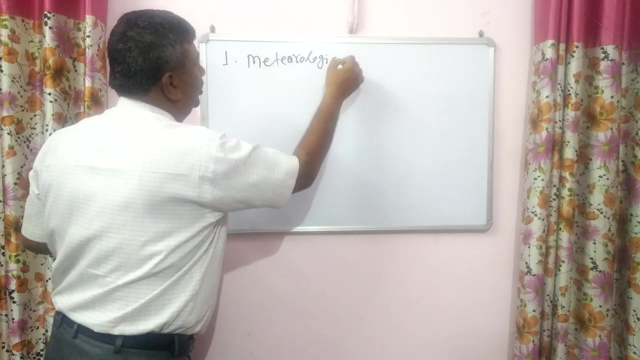 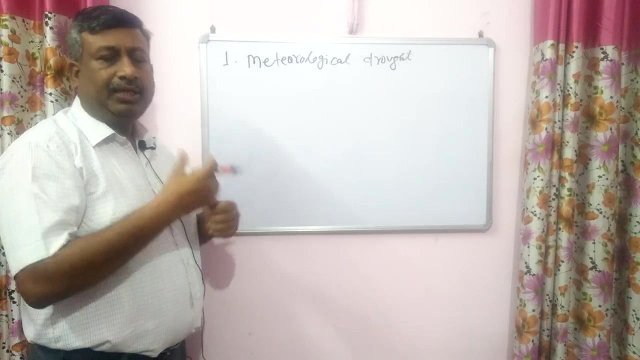 in this lecture we will discuss the different type of drought. So there are generally four types of drought when we talk about it. So first one is meteorological drought and it is related with the amount of rainfall received, Whether amount is deficient in a particular 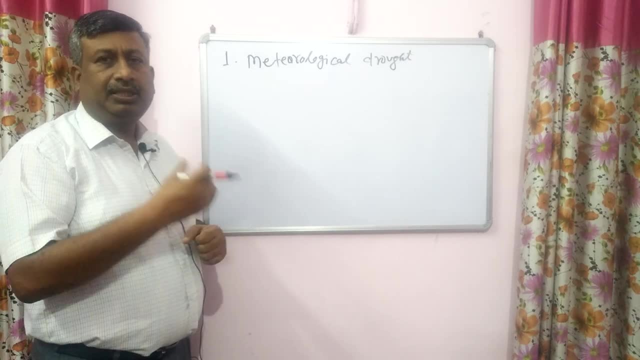 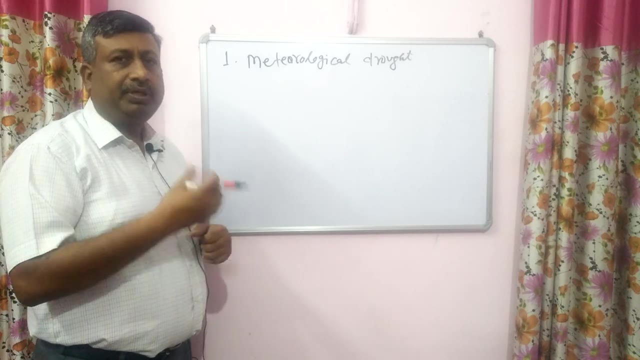 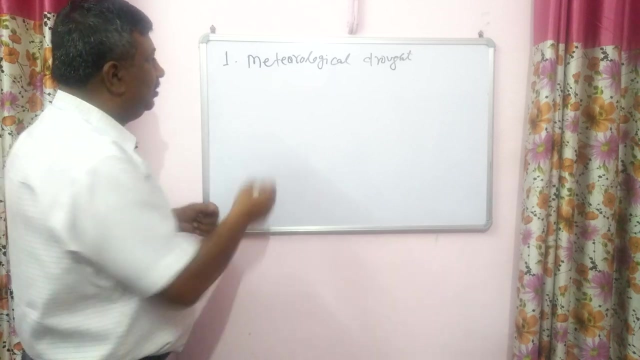 year, then that condition is termed as meteorological drought. So it is related with the meteorological condition. Second is rainfall quantity. So if the quantity of rainfall is less than a particular level, then it is said to be meteorological drought. So Indian meteorological department described. 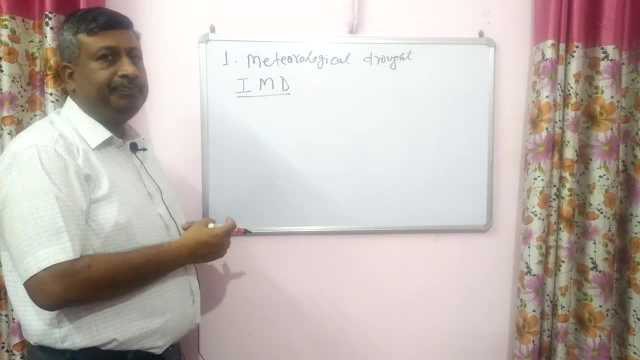 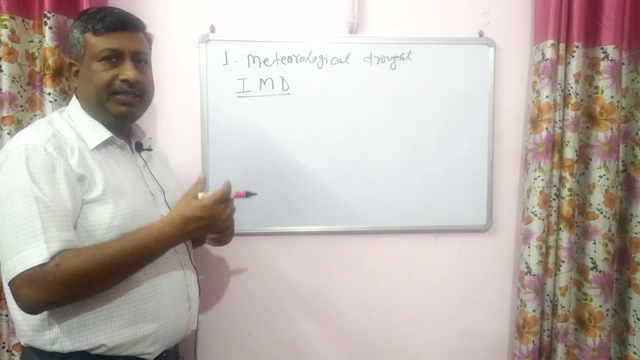 this meteorological drought. What do we call meteorological drought? First of all, a long average of rainfall is taken for a region or a country. For example, in our country, in India, this long average is 1193.. 1193.. 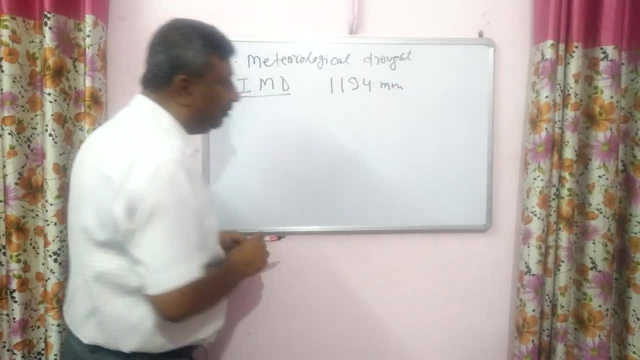 1193.. 1398, 1194.. 1198.. 11ổ, 1184.. 14경 15, Page Alex 1188.. 14, 9 0, 6, 7, 5, 8, 7, 8. 9, 10, 20, 21, 22, 27, 23, 24, 25, 28, 29, 30, 26, 33, 34, 35, 4, 34, 36, 37, 36, 38, 38, 39, 42, 42. 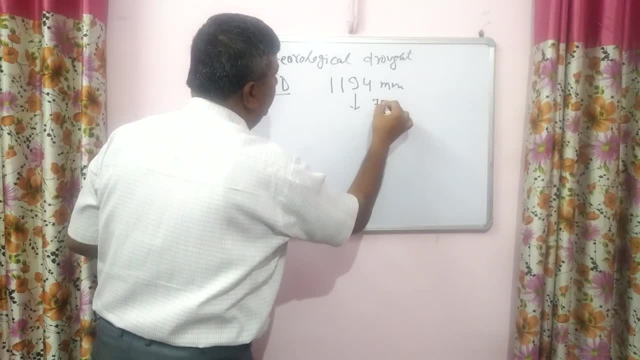 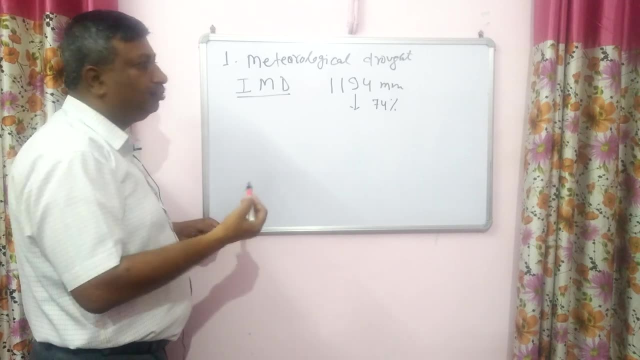 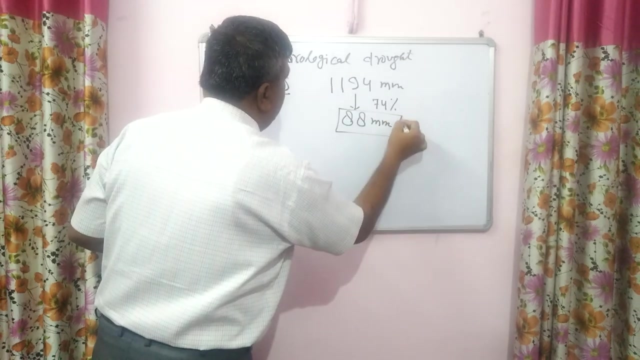 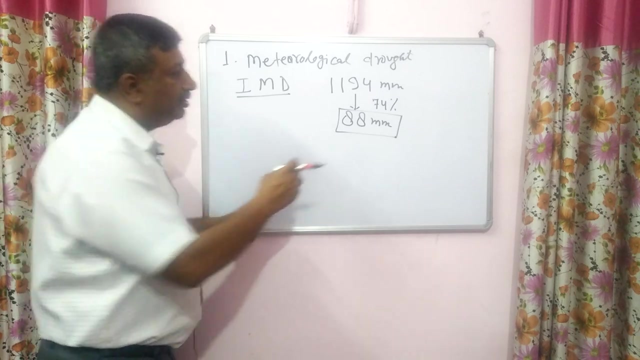 43, 44, 45, 54, 16, 76, 77. 73% rainfall is received in monsoon season, that is, June to September, and it is about 88 mm. So 88 mm taken as a reference by IMD, India Meteorological Department, 88 mm, sorry cm. it is 880 mm. it will be 88 cm. then 880 mm rainfall is considered as summer rain, which we consider as monsoon rain in our country. if it reduces rainfall by 25%, then it is considered up to the normal rainfall. it is not considered as deficient. 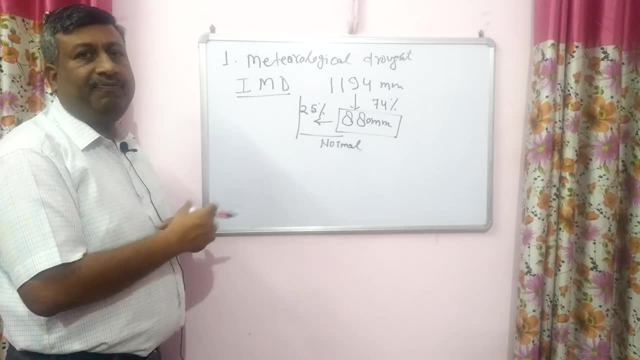 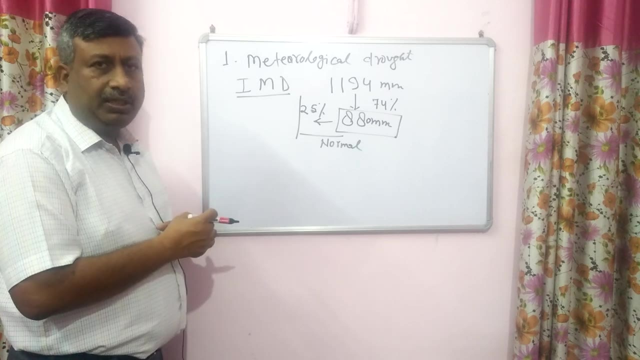 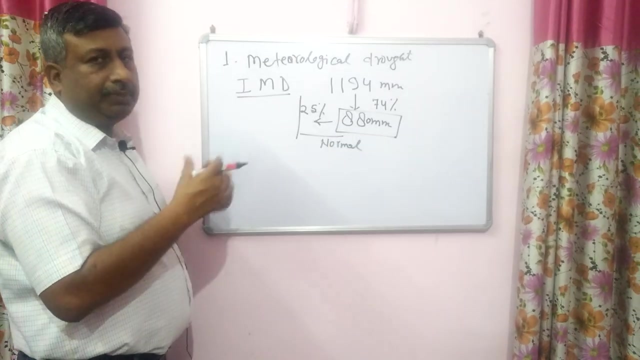 If rainfall is 880 mm, then it is considered up to the normal rainfall. it is not considered as deficient. If it is more than 25%, then it is considered as deficient and it is said to be metallurgical drought. So it means up to the. if we take 75% of it, then we will not consider it as drought condition. 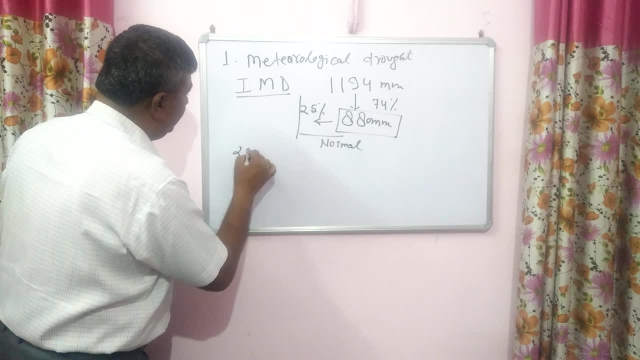 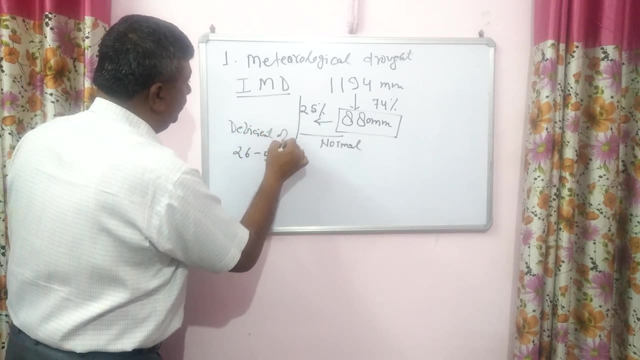 And if it is 26 to 50% deficient deficient of this 880 mm, then it is considered as drought. So if it is more than 25%, then it is considered as deficient and it is said to be metallurgical drought. If it is more than 2 to 5% deficient than we consider it as drought condition. it is considered a medianın pity and it is not dever. So if we took this above of 880 mm, then it is considered as moderate drought. 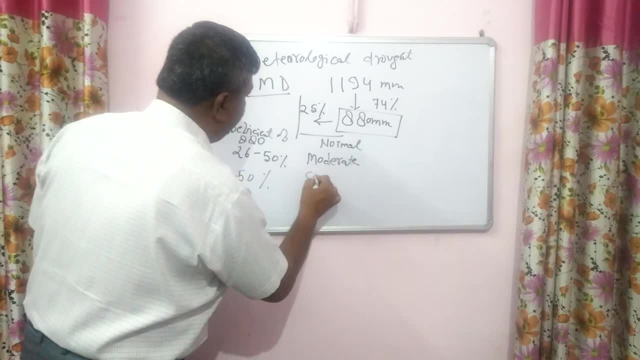 And if it is more than 50% deficient, then it is considered as severe drought. So this is definition given by IMD. What is drought So per year, if growth is largen on spring? yearhhhh sı also séc200€. 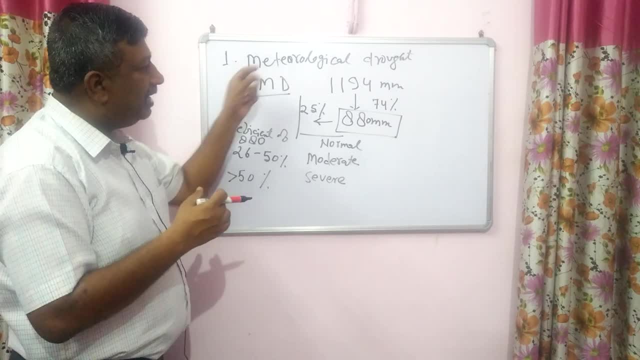 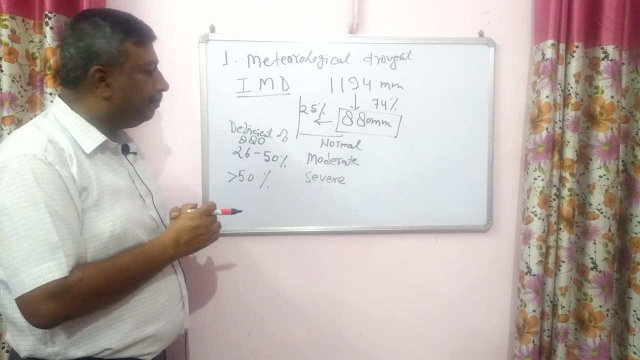 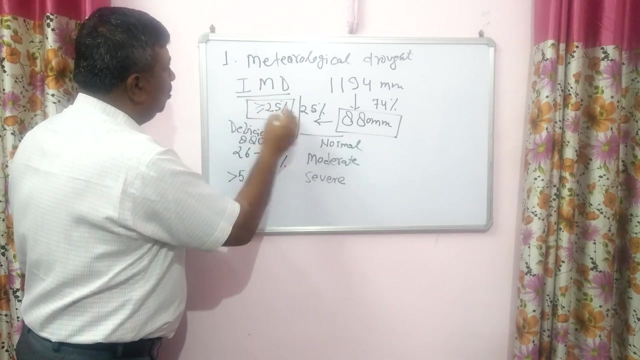 Then we take AM 7.. We take AM 7.. Then there is 30% percent average rainfall. come with a hair up to the 25 percent to school drop. many managerial metrological doctor considered new yoga. if it is more than 25 percent, then it is considered under drought. more than 25 percent, which is 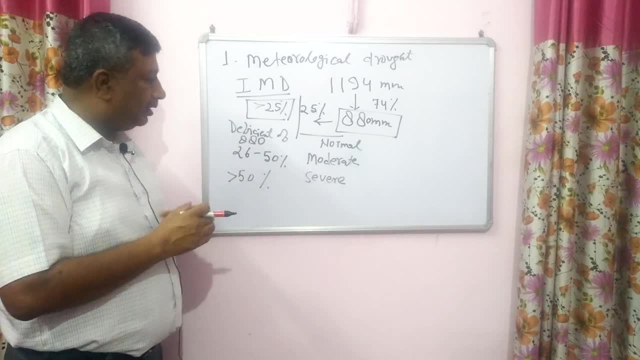 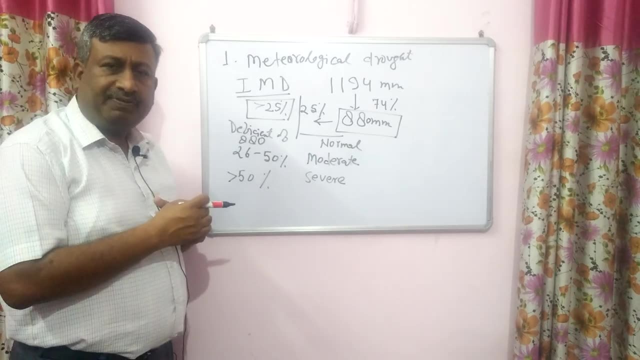 limit between 26 to 50, then it is said to be moderate drought, and more than 50 percent, then it is considered as severe drought. to kissy will locality killier. I'm kaka long average de na parega Ketanah a of. it was percentage say hum. 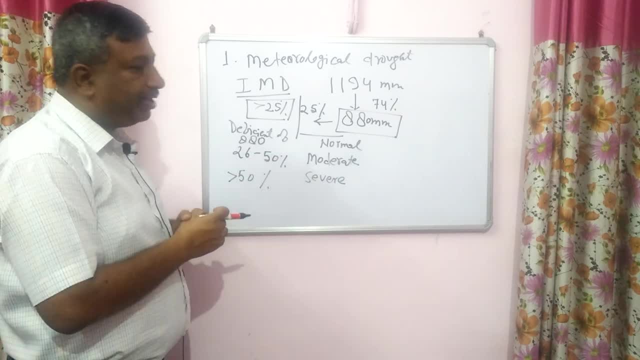 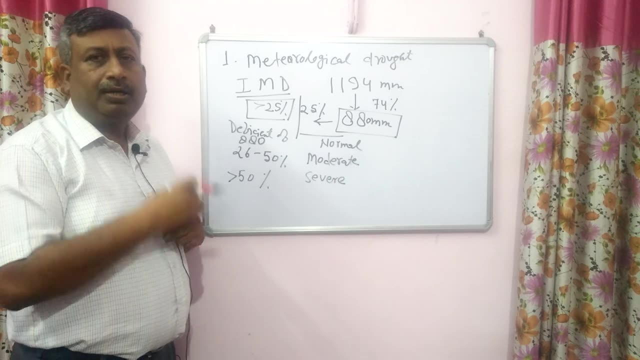 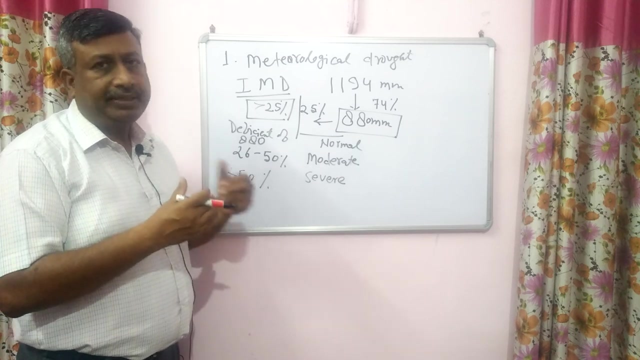 consider curcetane. he met a logical drought: severe, hey yeah, moderate. but for a country hole as a whole, keep puri country met dropped. who are here? no, hewager, I'm country clear hamper. consider curry: a pura area money for a country co-in dea May is salt drottier tie and I think our yeah Kittes all. 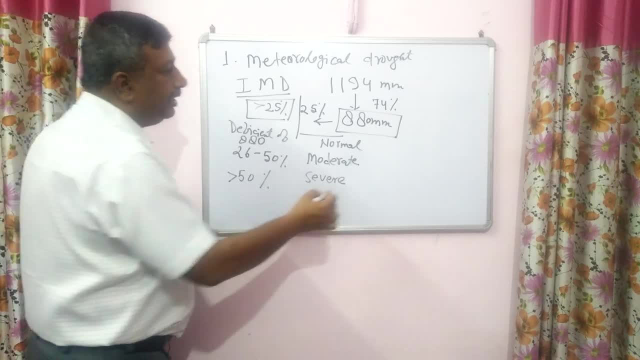 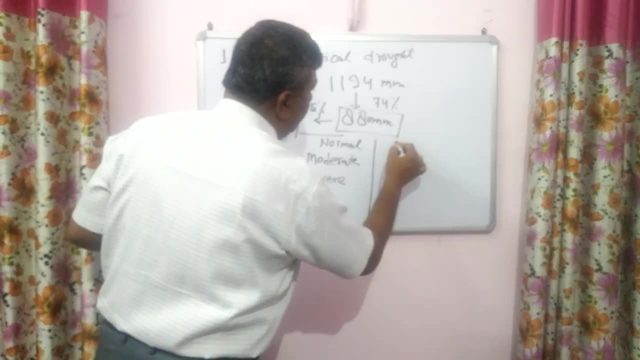 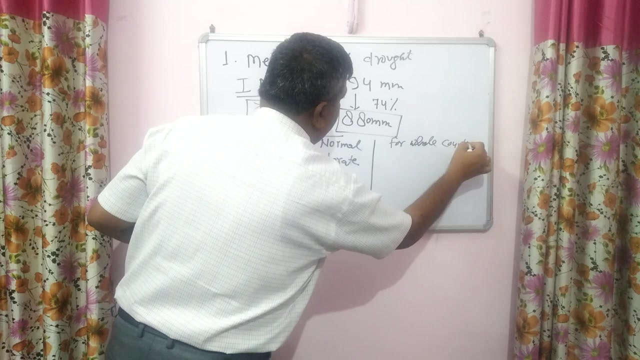 pellet drottier thaw, this year come drottier money G, then they are two parameters: particular year as a drought year, for country, for whole country. I am writing it here for whole country. if we consider drought less, then this parameter is not followed for whole country. 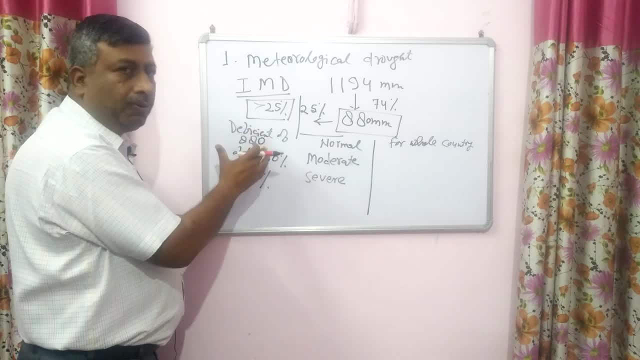 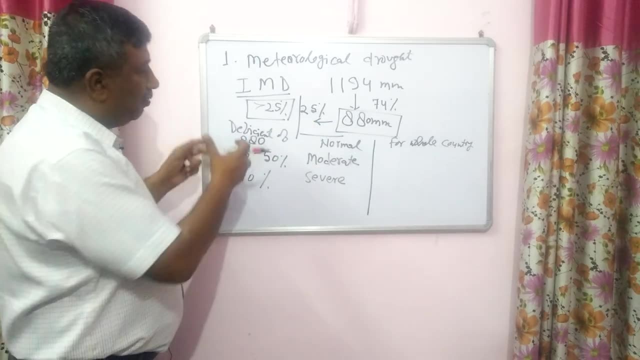 it is followed for particular region, particular area, particular district, that what is long term average. I have taken its example of that locality, of that district and if there is deficiency due to this, then it is a meteorological drought. but in whole country, if we consider 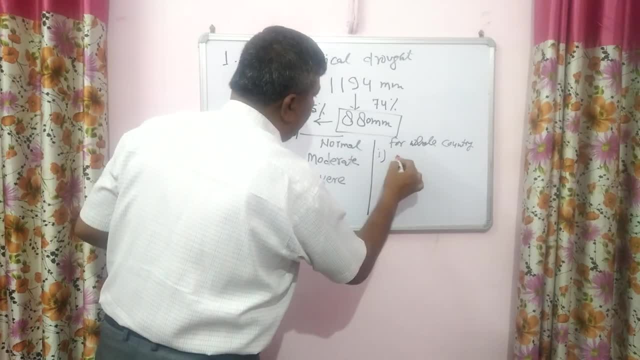 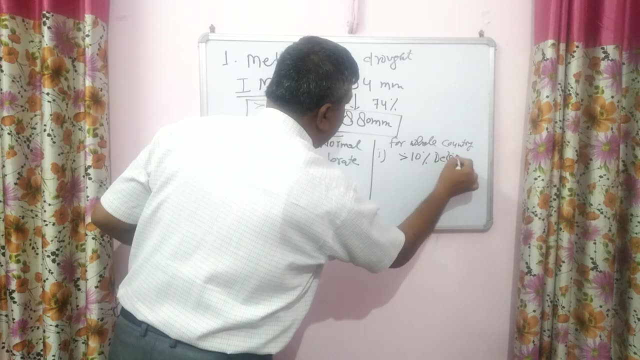 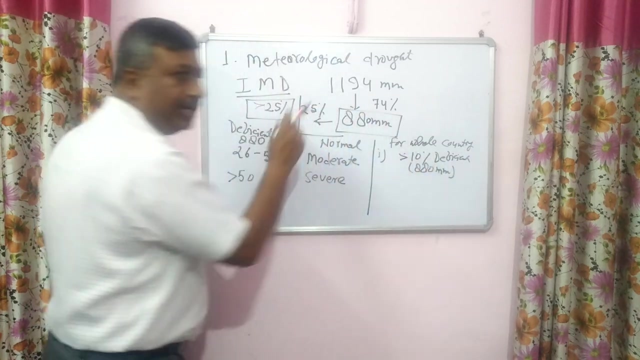 whole country. then there are two parameters. number one: rainfall should be more than 10% deficient. the rainfall of this 880 mm for whole country. we are talking, so we will take 880 mm. if we are talking about this, then it will be different for a particular area. 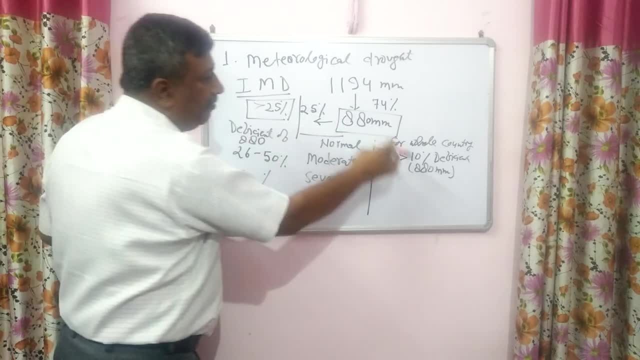 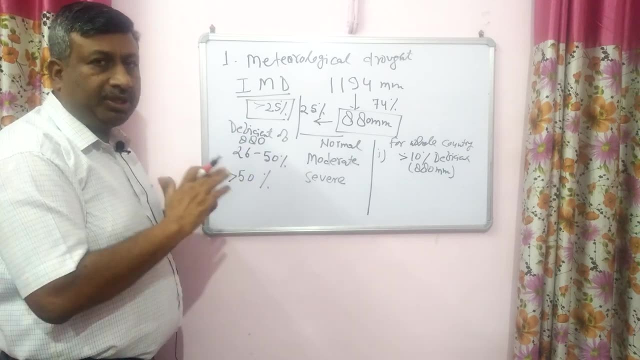 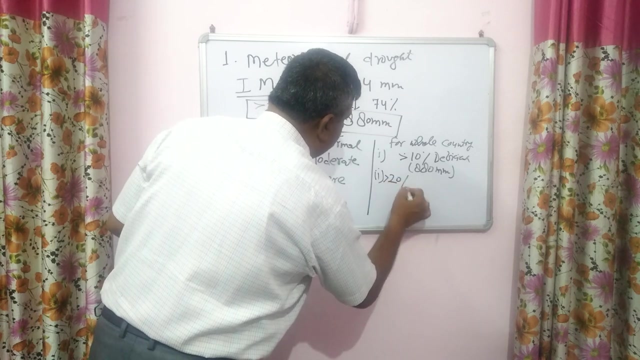 this value will be different For every area it will be different, but for country this 880 mm is considered. So the rainfall there should be more than 10%. it should be deficient. Second, it should be the area more than 20% area of country should be should have more. 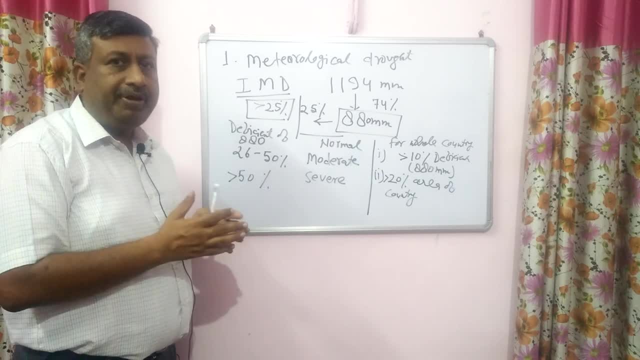 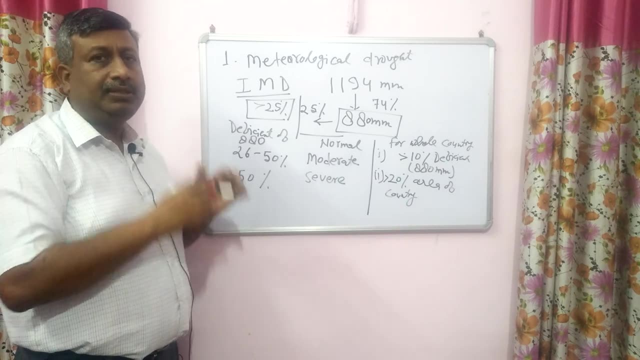 than 10% deficient rainfall. if in country in 20% area the deficiency of rainfall is more than 10%, then that particular year is considered as drought year. So it is important for you to understand that we will say meteorological drought when we 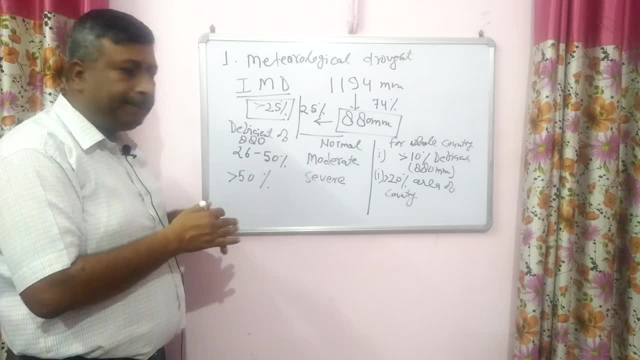 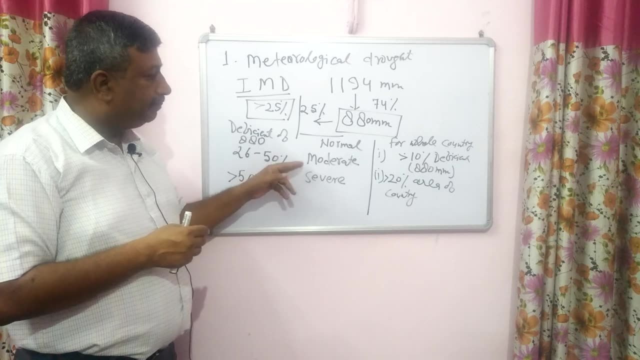 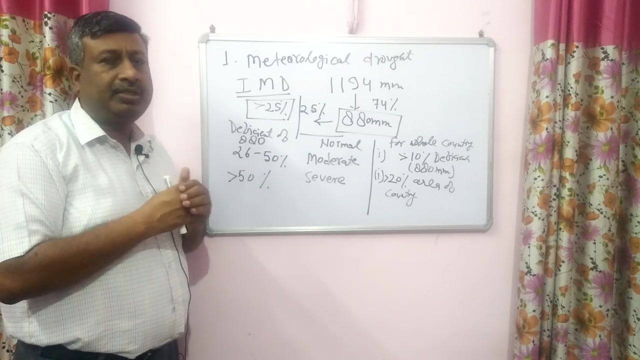 take long average rainfall and if it is more than 25% then it is meteorological drought, and if it is 26 to 50% then it will be in the condition of moderate drought and more than 50% then severe drought. So this particular we can take out for any particular district because that district 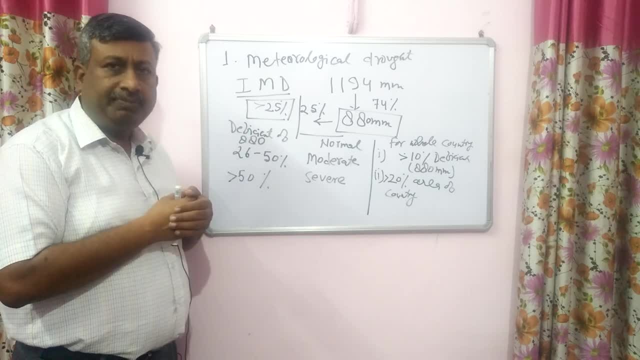 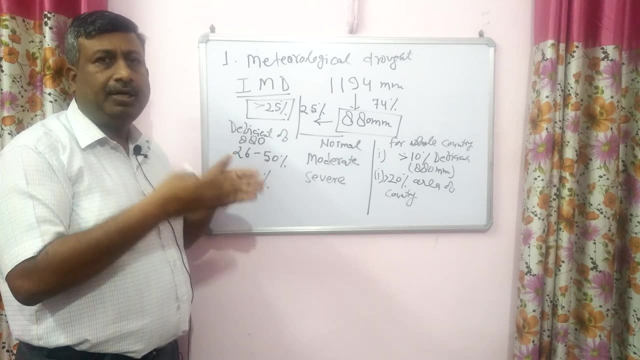 has average rainfall. we can take out for any particular city. we can take out for any particular city that this drought year will come or will not come. there is no meteorological drought or not. So there, we can take out the average rainfall of the city, the average of long time, and we 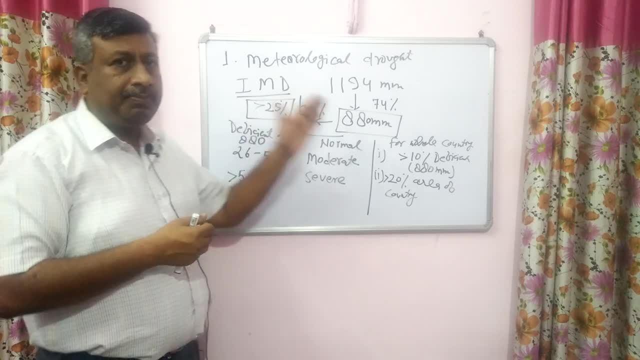 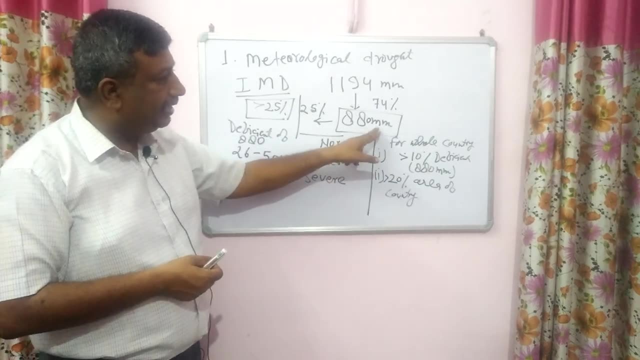 can see if there is any deficiency or not, But if we talk about the country, then for the country there should be more than 10% deficiency in rainfall and for that, 880 mm is considered If there is less than 10% of this rainfall. Then the average of this city should be more than 10%, and if the main reason is that there is more than 10% of this city is affected, then it is considered as meteorological drought or drought year. So meteorological drought is related with the less amount of rainfall. 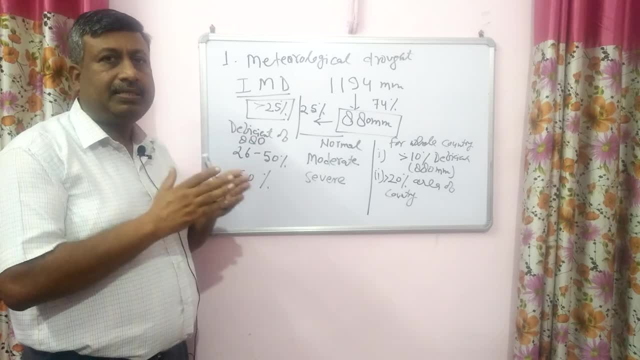 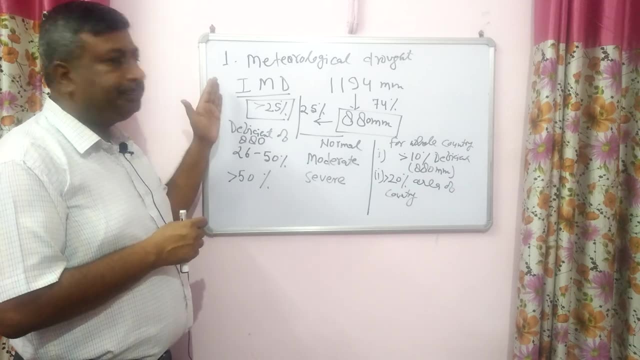 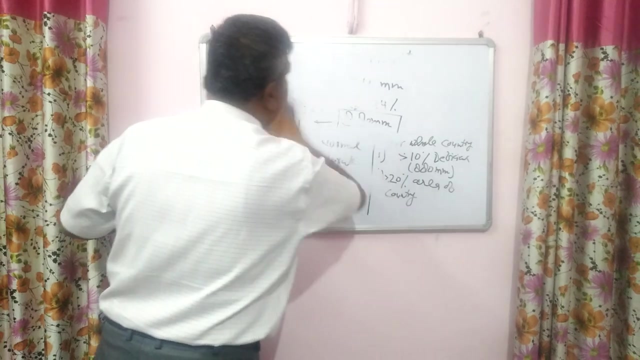 So this was about the meteorological drought and drought year and it is classified as meteorological drought. So let us see what is the next question, And it is classified by IMD: Another advancement in drought. if we see in sequence the condition after metallurgical drought, that is agricultural drought. 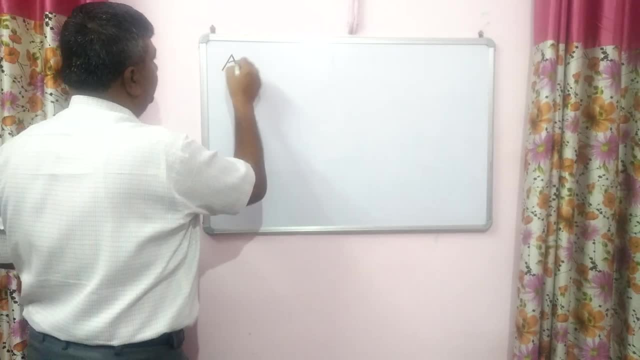 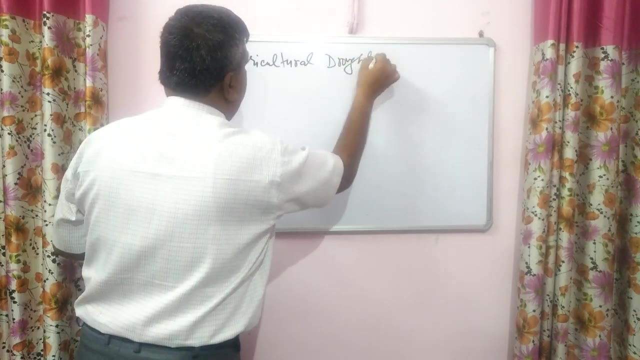 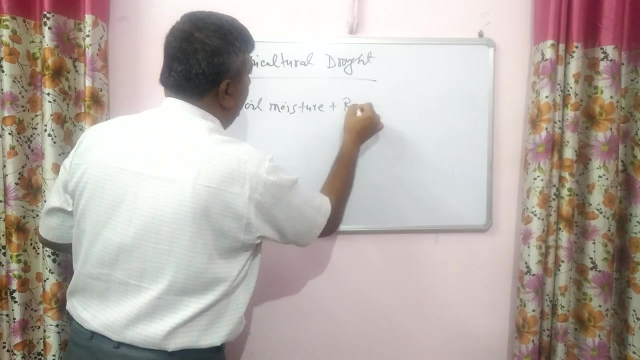 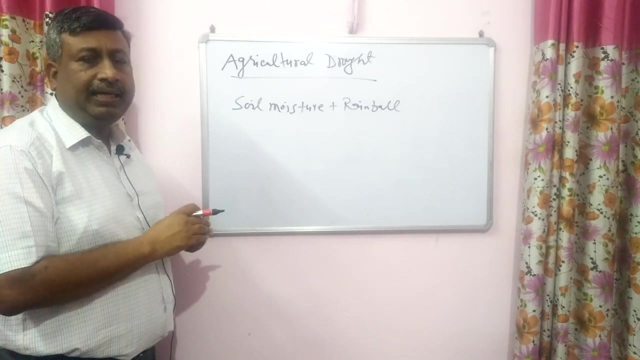 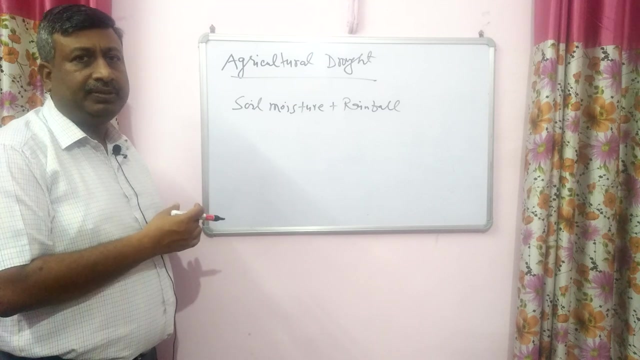 In case of agricultural drought- here crop growth is concerned- The soil moisture and rainfall are not sufficient to fulfill the plant water requirement, that condition is considered as agricultural drought. When the amount of soil moisture and rainfall is not enough to fulfill the plant water requirement for its good growth, then it is considered as agricultural drought. 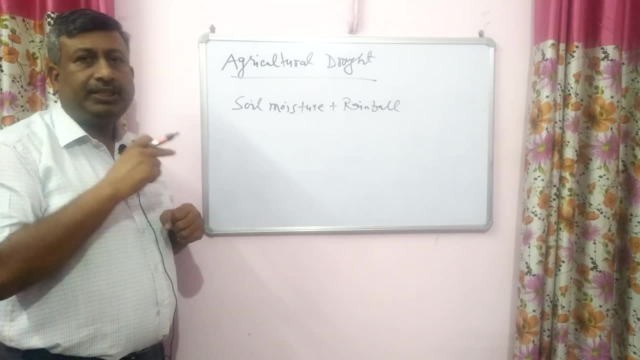 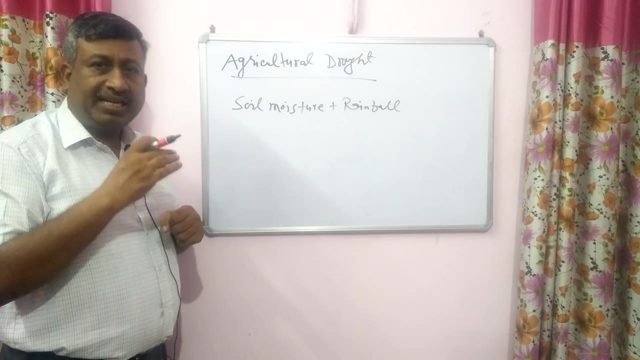 It is not like that In case of metallurgical drought. amount of quantification is given: 26 to 50 percent, more than 50 percent and national average 880 mm. more than 10 percent and 20 percent area affected. 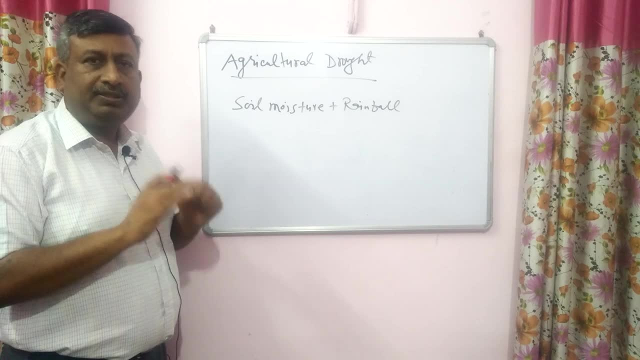 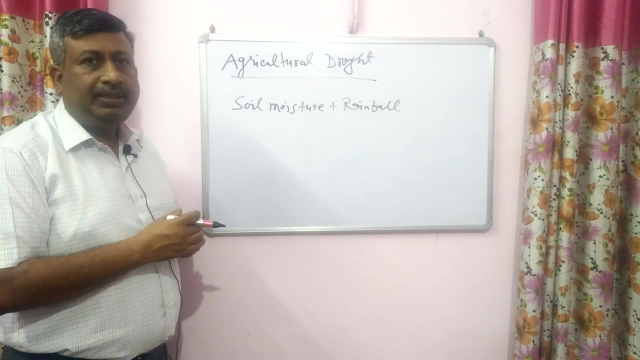 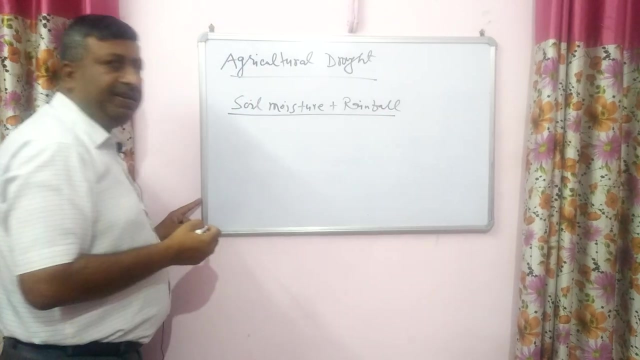 But in case of agricultural drought, there is no quantification, there is no limit, Simple term. when soil moisture plus rainfall quantity is not sufficient to fulfill the plant water requirement, then this condition is known as agricultural drought. And this This condition vary from crop to crop. 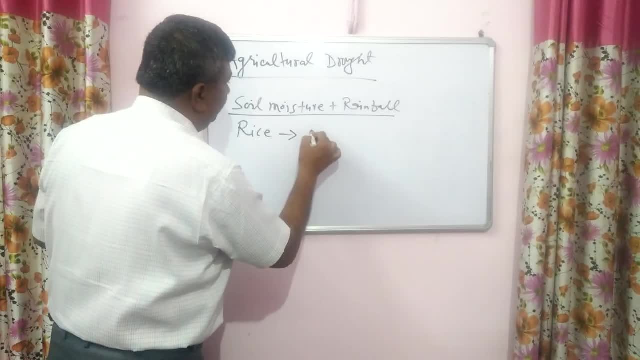 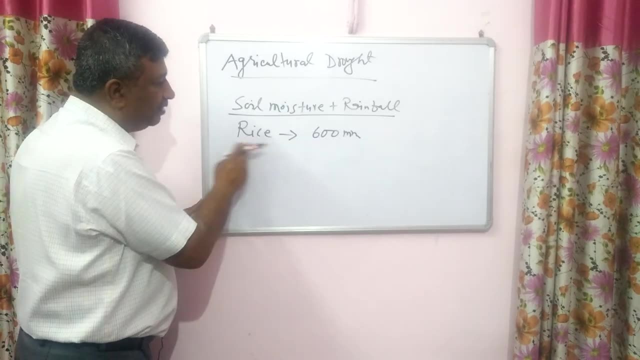 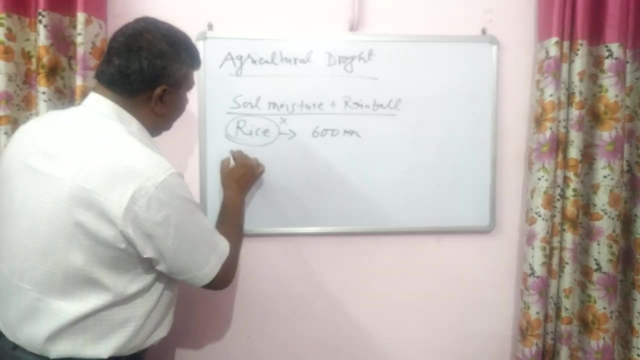 For example in rice Rice. In case of rice, 600 mm water is through soil moisture plus rainfall and this amount is not sufficient to fulfill the water requirement of rice, Then this is agricultural drought for rice. But this 600 mm is sufficient for maize, pearl, millet and sorghum. 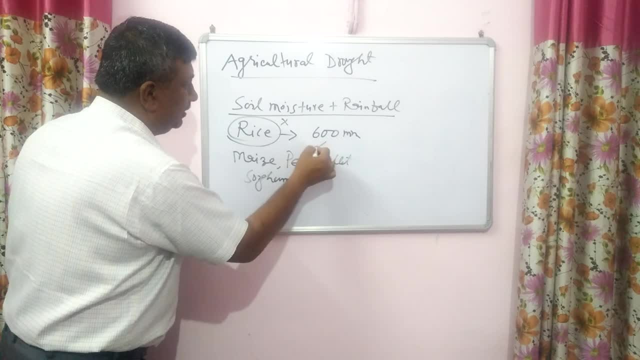 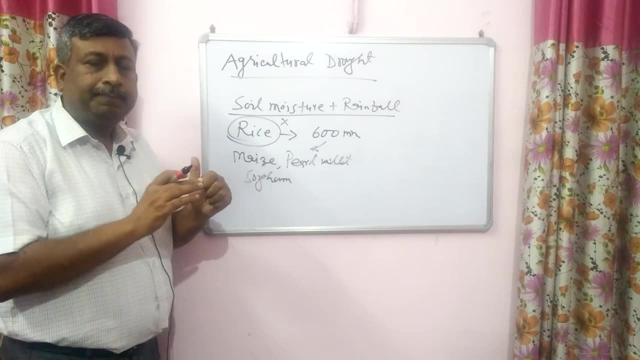 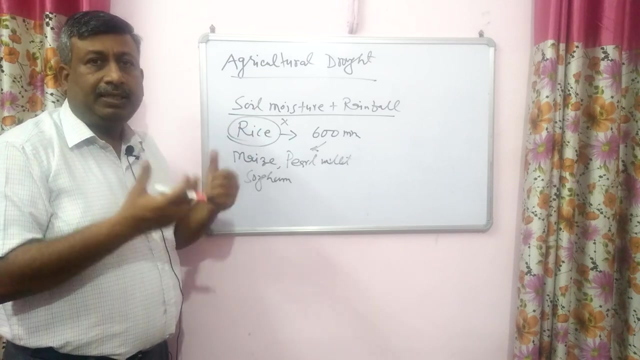 And for this crop this quantity is sufficient, Then for this crop there is no agricultural drought. But for rice it is drought. It means it depends upon the nature of the crop. Number one, Number two: soil characteristics. If soil can hold more moisture, then there is less chances of agricultural drought. 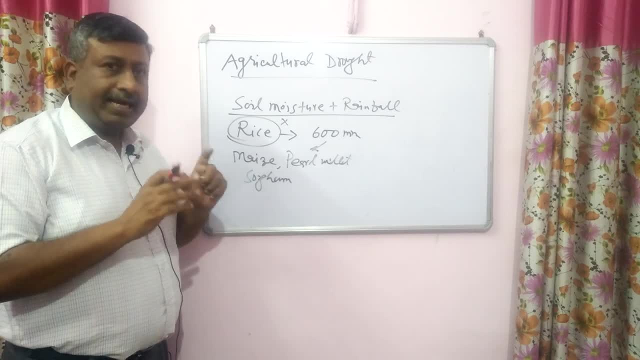 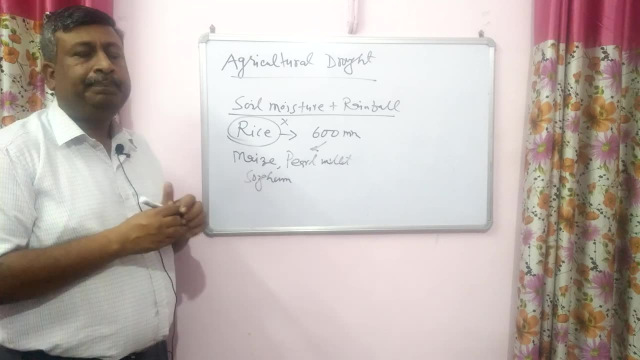 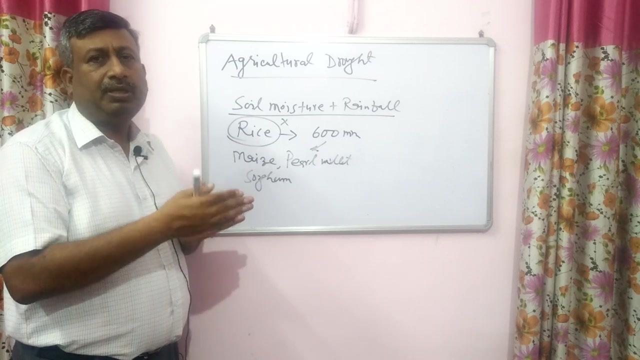 So there is no quantification, It is just the case of water moisture available And plant water requirement. So here we have to understand agricultural drought. When soil moisture and rainfall is not sufficient to fulfill the plant water requirement, then we call it agricultural drought. 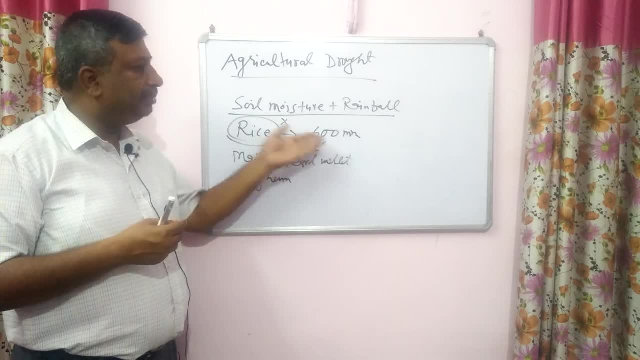 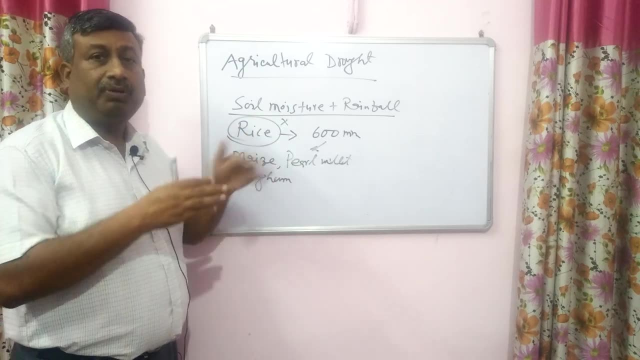 Now water requirement for rice is very high, So 600 mm is not able to fulfill the water requirement. So in that case there is drought for rice. But for maize, pearl, millet and sorghum water is very sufficient. 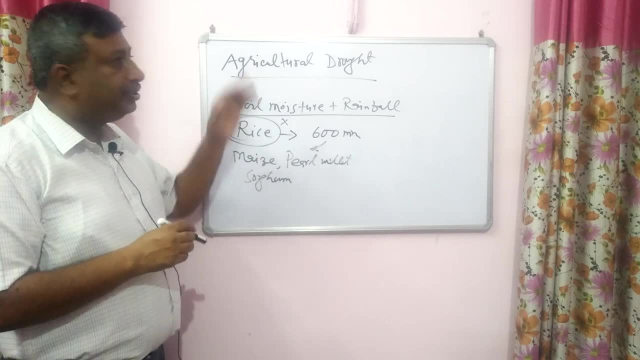 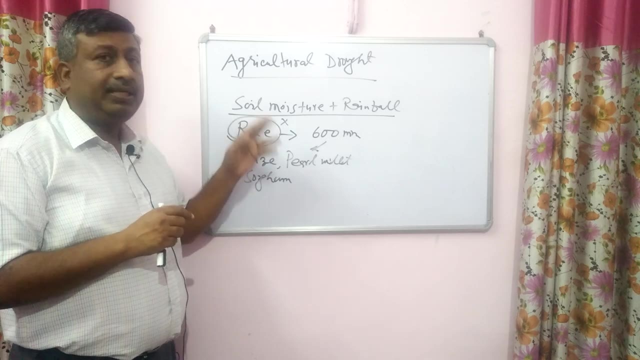 So there is no drought for that. So this agricultural drought depends upon many factors. Number one is type of crop. Number two The crop to be grown. Which crop is being grown? Number one, Number two: Soil characteristics, Because rainfall can hold more moisture. So it can supply more moisture. In some soils there is more runoff, Like clay soil vertisol, So it will not be able to retain moisture. Second: frequency of dry period. How much dry spell is coming Then? erratic behavior of monsoon. 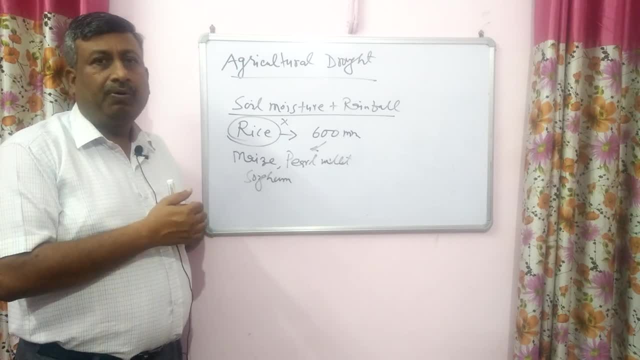 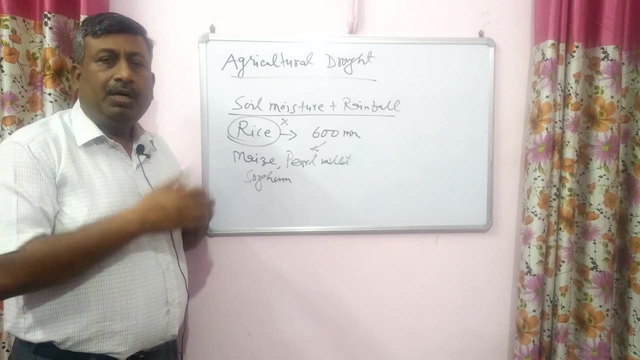 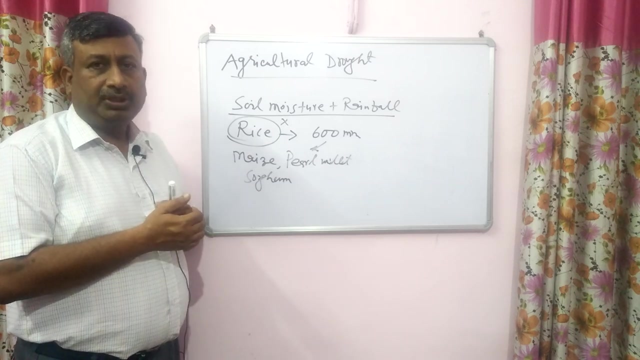 If monsoon is late or early, withdraw, So there are chances of agricultural drought. So this agriculture drought is related with the erratic behavior of monsoon, crop and soil characteristics. So if the frequency of dry spell is high, then the chances of agriculture drought is high. 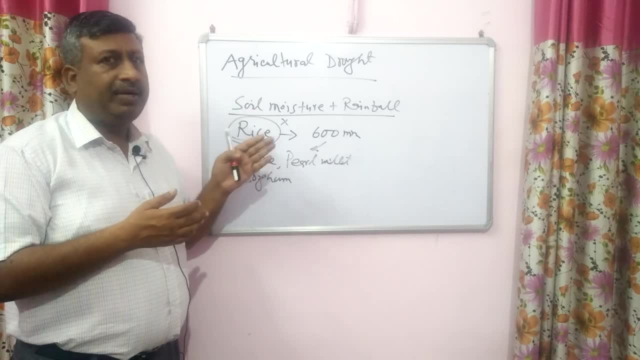 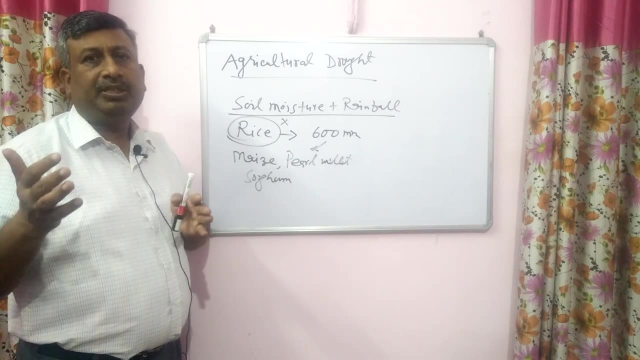 So arid and semi-arid area, There are more chances of agriculture drought because of dry spell. Dry period occurs In the beginning, the rainfall is good. There is no rainfall in the middle. Then there is a rainfall in the late season. Sometimes monsoon comes very late, So agriculture drought occurs. Dry period occurs In the early period. the crop's water requirement cannot be fulfilled. So agriculture drought is a relative term. For one crop there can be agriculture drought, But it cannot be for the other crop. 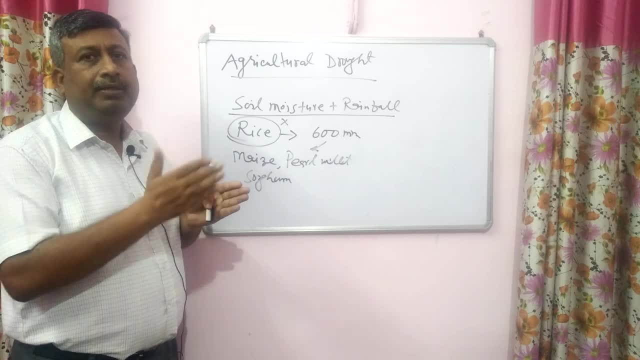 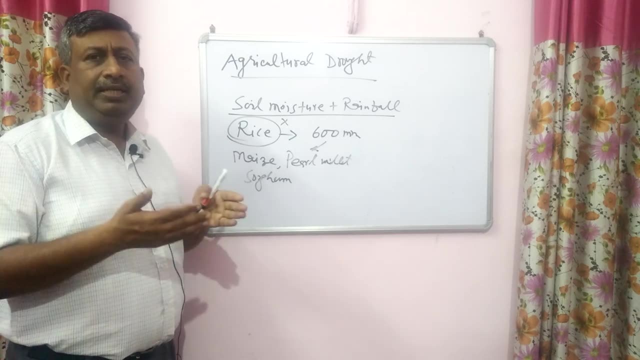 So for those who have more water requirement there can be agriculture drought, But it cannot be for less. But suppose the moisture ability is very low. It is 300 mm, And 300 mm quantity is not sufficient to fulfill the water requirement of any crop. 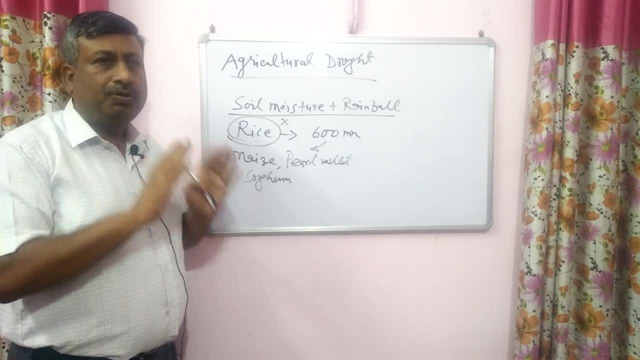 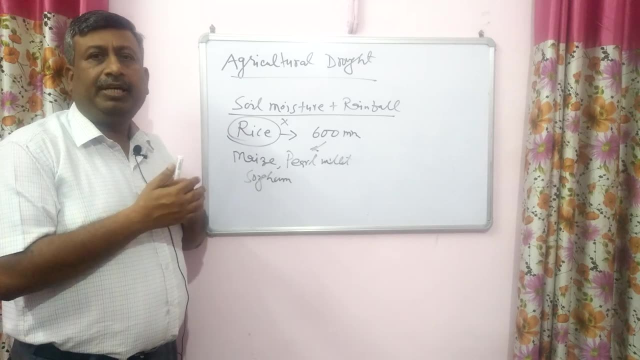 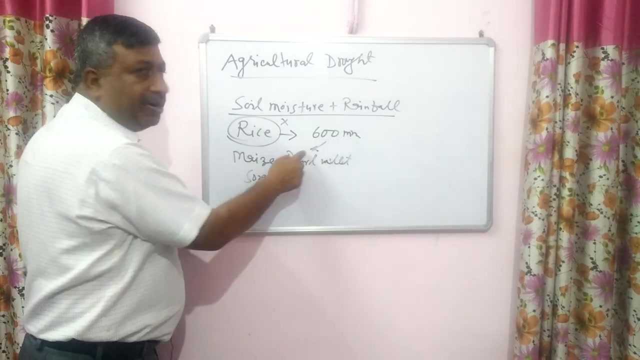 So in this case, agriculture, drought is for all crops. So the next condition is meteorological drought. Why? Because of the insufficient rainfall, Because there is a deficiency- More than 25%. rainfall is decreasing. When rainfall will decrease, then what will happen to the crop's water requirement? 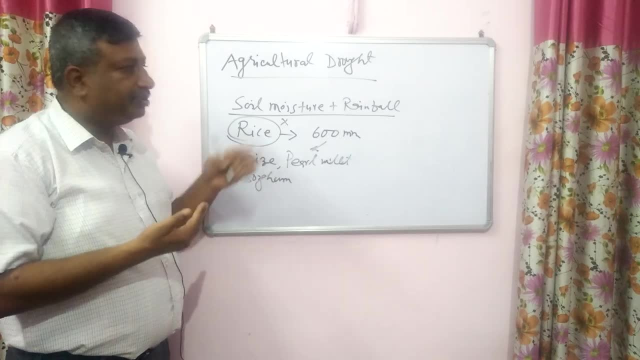 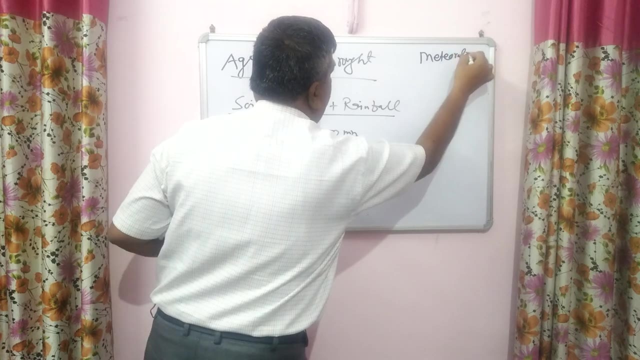 Water requirement is that much, But its demand plant will not be able to be fulfilled. So first there will be meteorological drought, After meteorological drought, the condition that will come. that condition exists Agricultural drought. So this is the sequence. 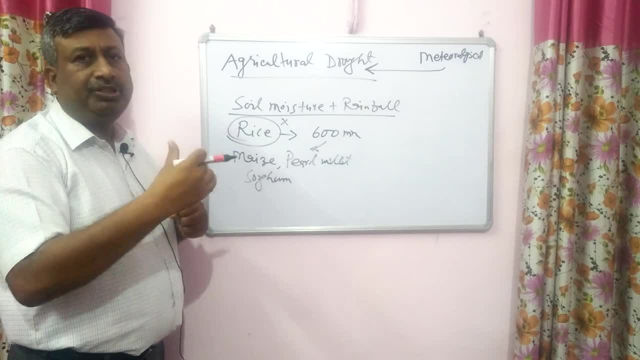 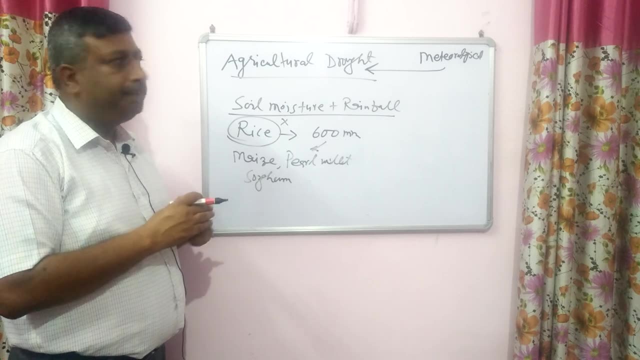 First of all you can ask for the sequence of the drought. So the first one is meteorological drought Because of insufficient rainfall, Deficiency of rainfall- And when there is a deficiency of rainfall then plant water requirement is not fulfilled. Then agricultural drought. 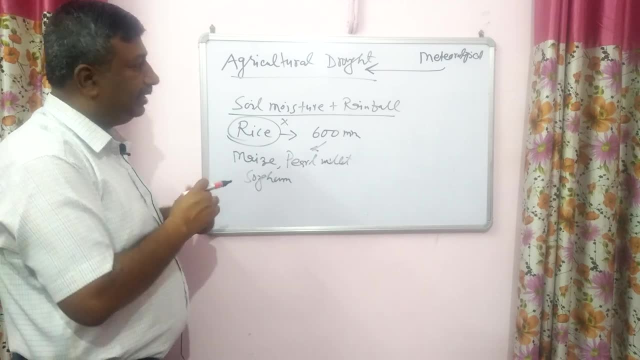 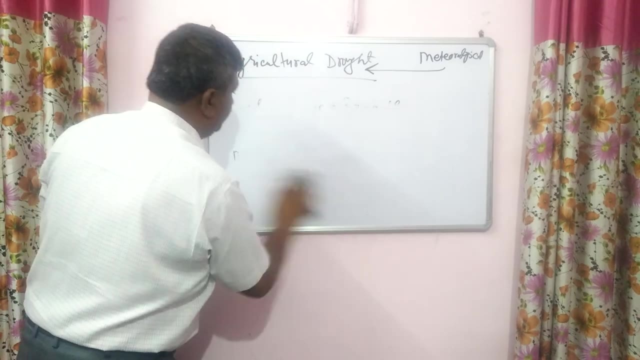 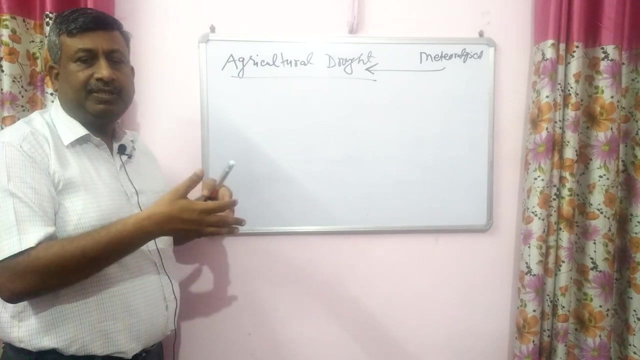 So this drought will come after this. Then, third one is hydrological drought. In case of hydrological drought, See. hydrological drought is related with the. hydrological drought is related with the water reservoir. Water is present in lakes, rivers, ponds. 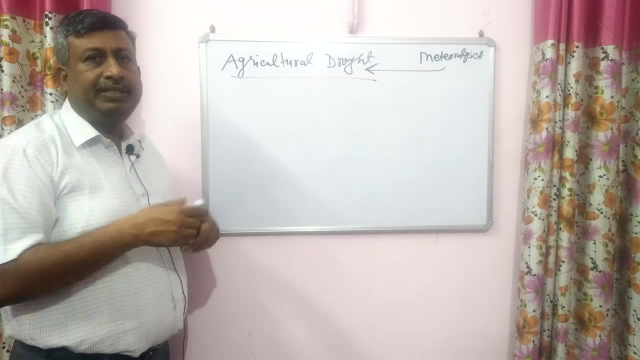 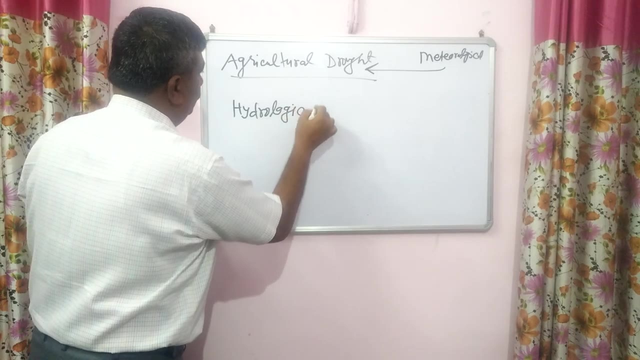 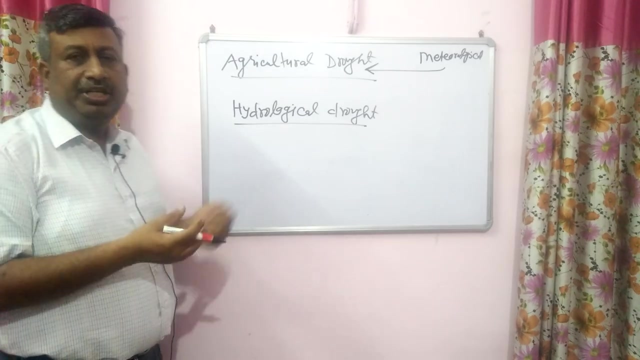 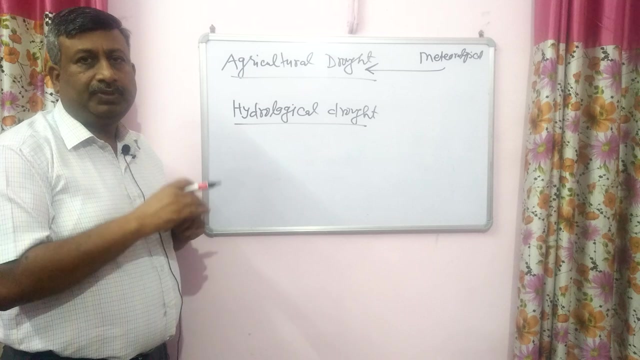 When water is deficient in water reservoir, then it is known as hydrological drought. Water is present in water bodies, surface water bodies and sub-surface soil, And most of the water is present on surface Lakes, rivers, ponds And when there is an insufficient rainfall. 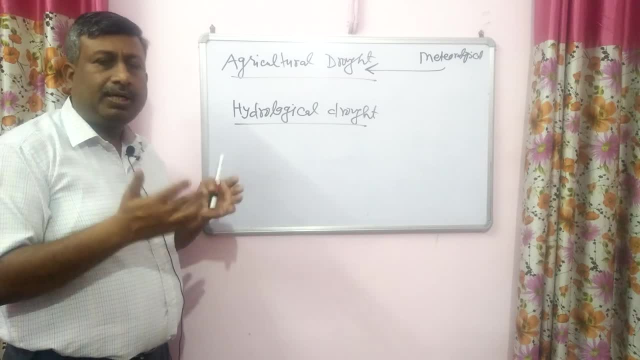 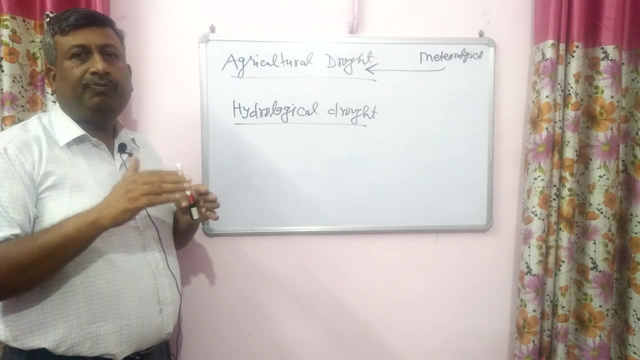 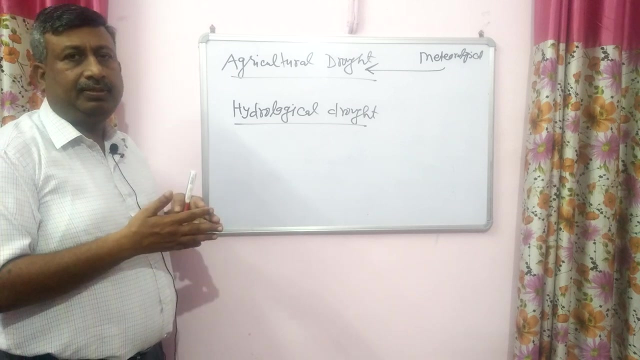 then the water that remains from the snowfall or the rainfall, or if this precipitation is less- either rainfall or snowfall- then water present in water bodies, lakes, ponds, rivers, wherever the water collect- then water starts to decline And water reaches. 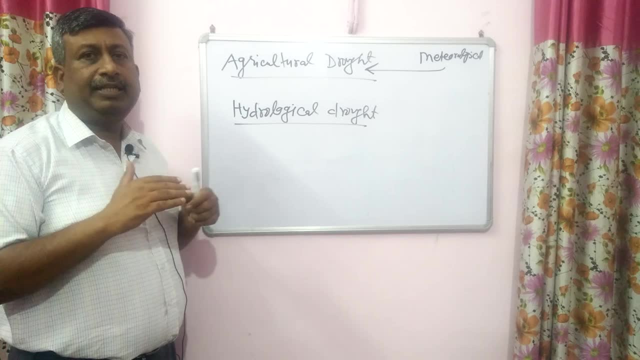 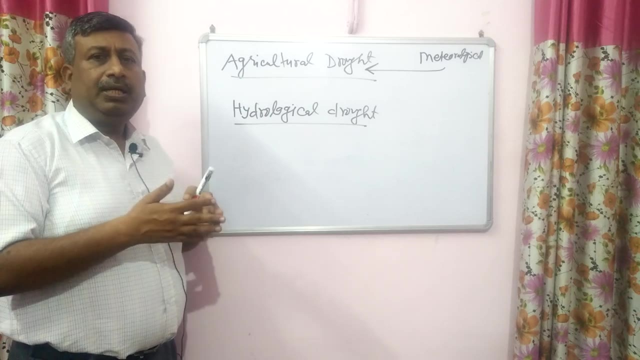 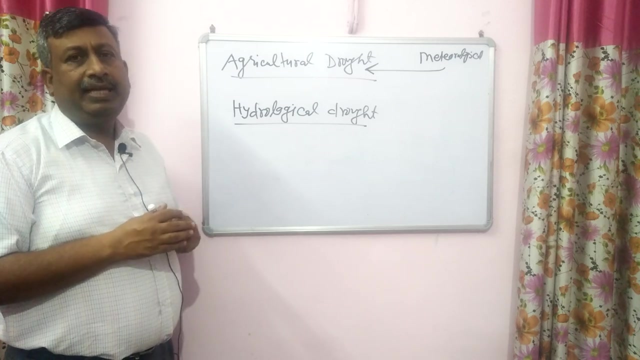 below a threshold level- critical level- then it is said to be hydrological drought. So what is hydrological drought? When in rivers, lakes, ponds, ponds water is below a critical level, a level below a threshold, that condition is termed as hydrological drought. 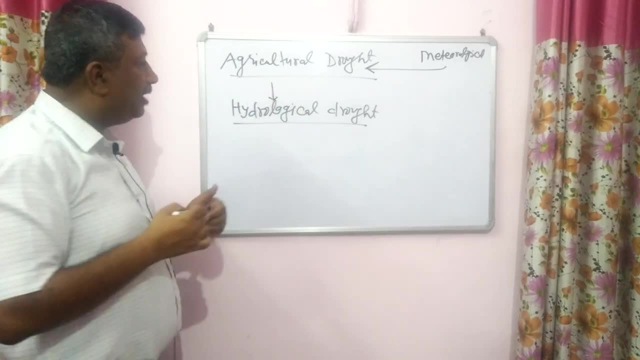 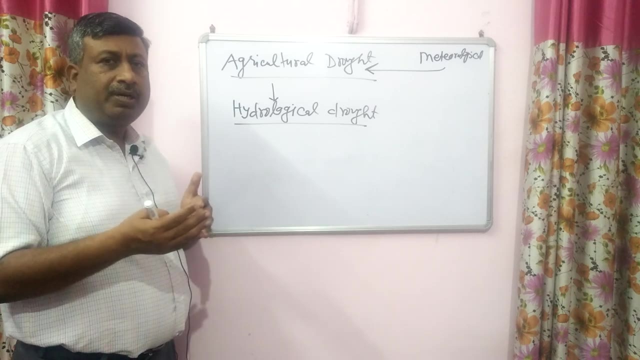 So the sequence that comes after agricultural drought, that is hydrological drought. So first one is metallurgical drought, Then agricultural drought And water starts to decrease a lot Water starts to decrease. in ponds Water is not available. That is hydrological drought. 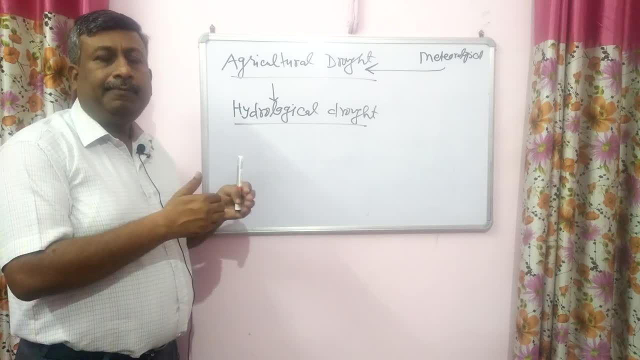 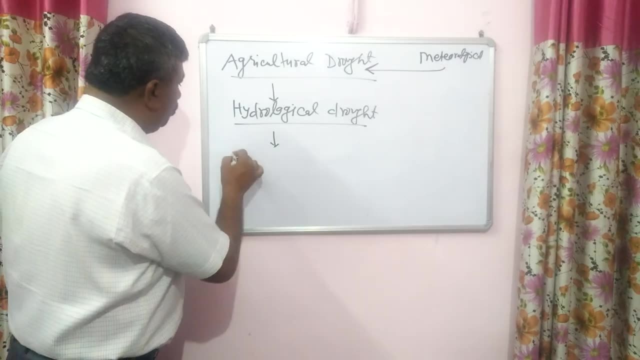 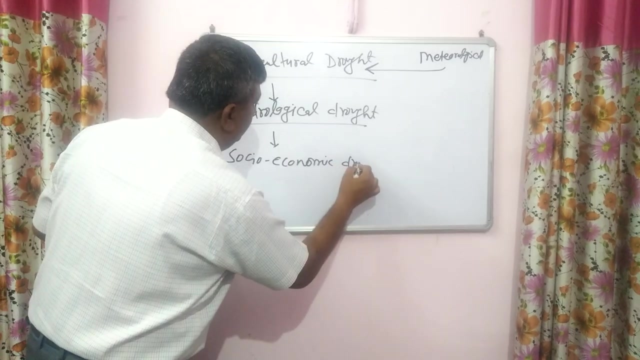 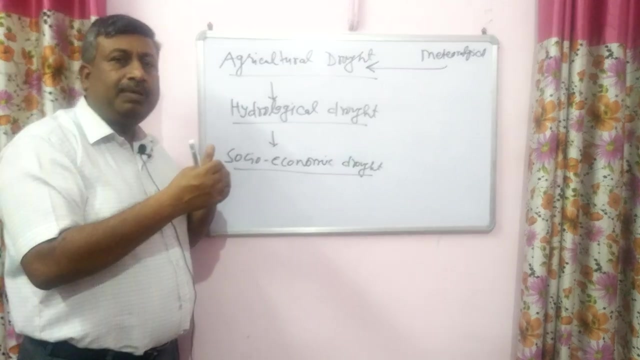 So what is hydrological drought? related to Amount of water present in water bodies, water reservoir. Then fourth one is related with the socio-economic drought. Socio-economic drought, This socio-economic drought is related with the society. Now see if the water in the river decreases. 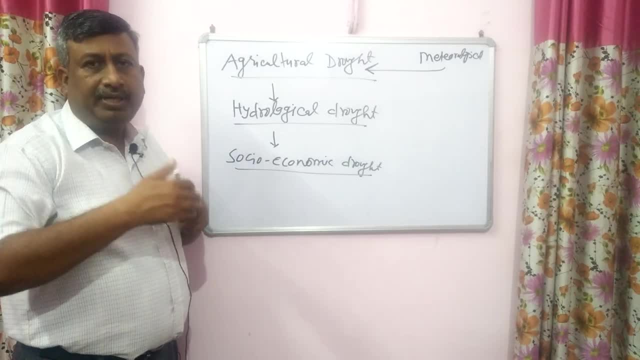 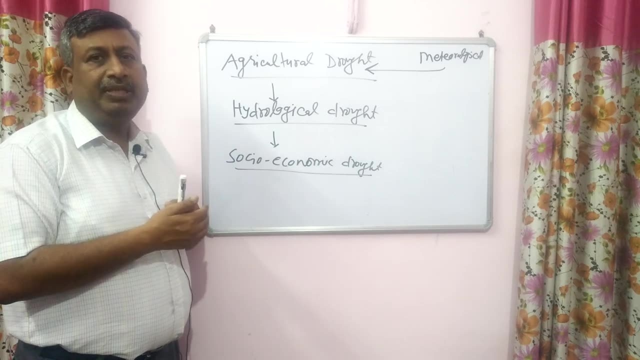 if the water in the lake decreases, then drinking water will decrease. The availability of water for the industry will decrease. These are hydro-power projects where electricity is being made from water. If there is no water in the reservoir, there is no electricity production. 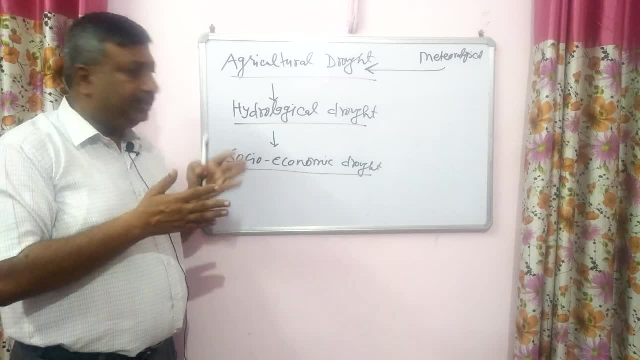 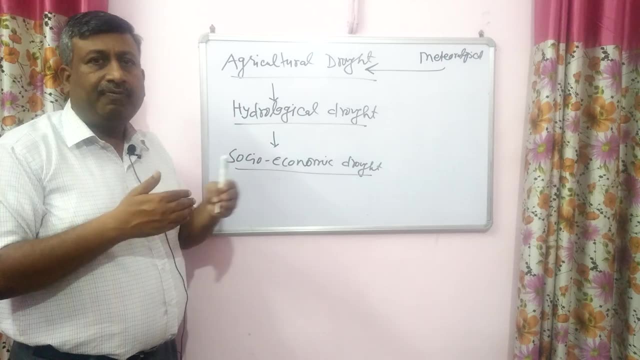 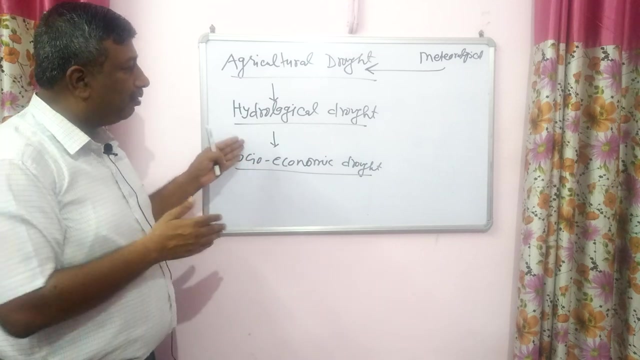 Then society is affected, Industry is affected And that when the quantity of water is so low that the work society, work or drinking water is affected, industry is affected, electricity is affected. then it is known as socio-economic drought. So this is the fourth condition of drought. 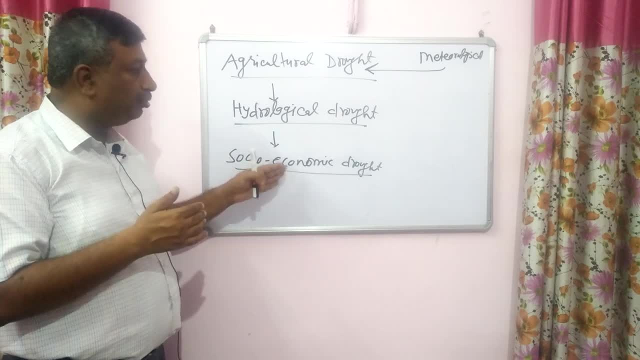 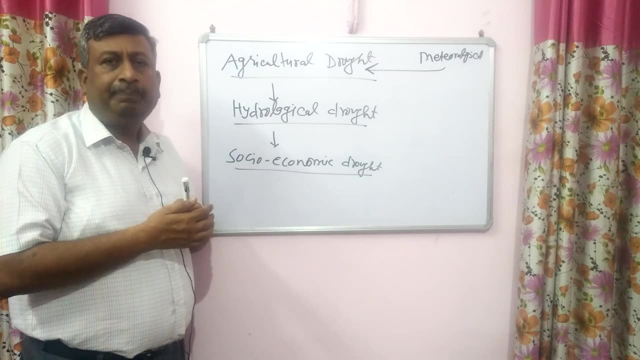 So first, metrological, agricultural, hydrological and socio-economic drought. So socio-economic drought is when the water in the reservoir is so low that it is not available to drink, the water is not available to run the industry, the water is not available to produce electricity. 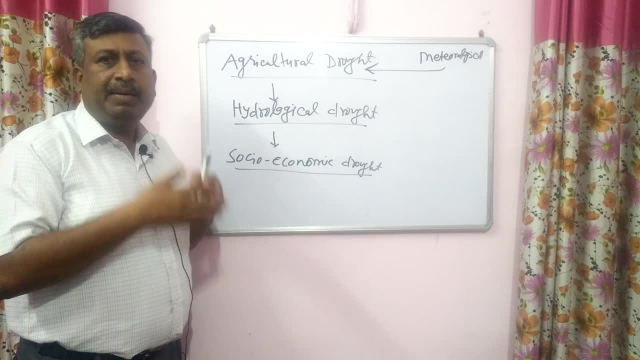 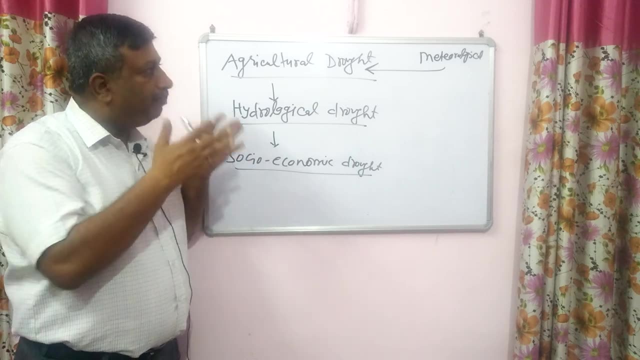 the reservoir is dry, the rivers are dry, the lakes are dry, the animals are not getting water. That condition is termed as socio-economic drought. These are the four kinds of droughts And the IMD of this is very important. Let me tell you again. What is a metrological drought? When it is more than 25% deficiency? again, understand this: more than 25% deficiency of long average of rainfall, The rainfall of any locality rainfall, and if there is a 25% air deficiency then it will be called a metrological dot. 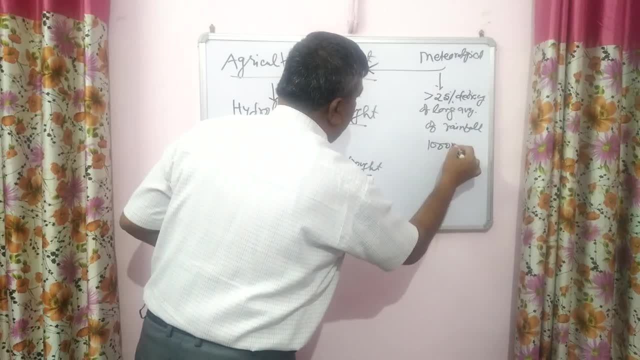 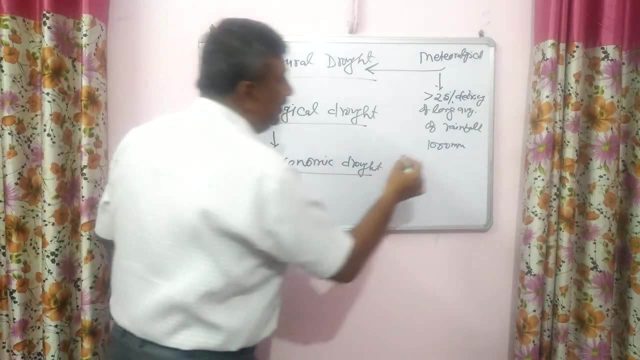 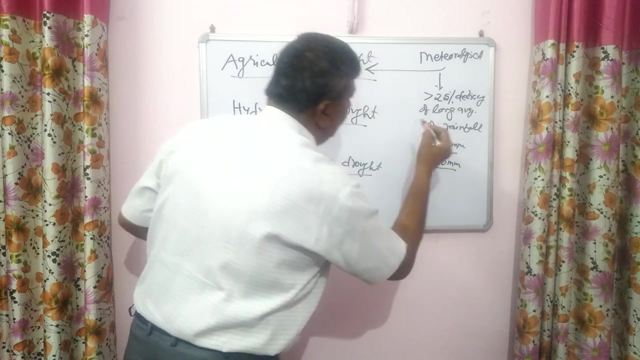 For example, for any city. suppose there is a 1000 mm rainfall average annual rainfall, so it is taken out in the long term average rainfall and suppose its 25% is 250 mm. If suppose there is a 700 mm rainfall, because 25% will be 250 mm, so it is more than 25%. 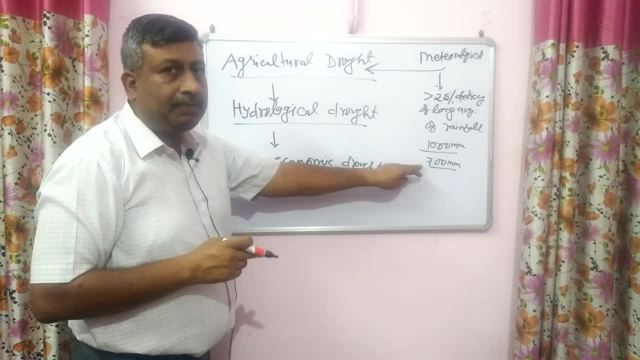 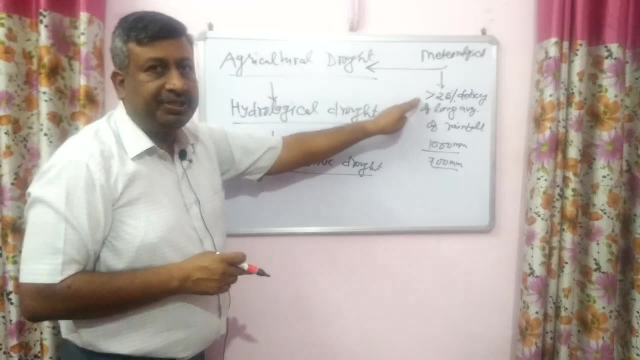 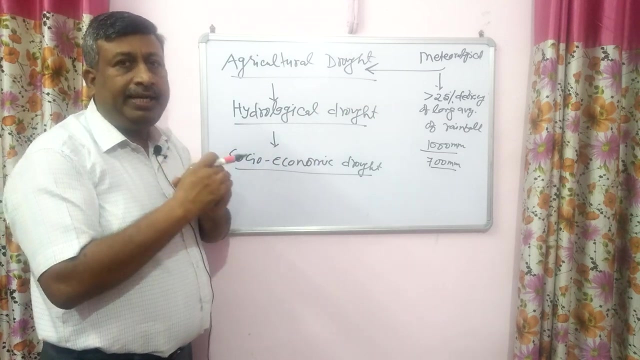 it is a reduction of 30%, then that city or that place is considered under a metrological dot. So you have to understand that for a metrological dot the quantification is fixed more than 25% of long average In our country, as I told you in the beginning, the Indian monsoon is 1194 mm in total. but 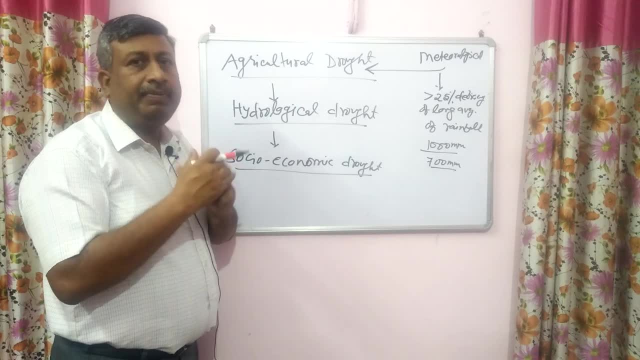 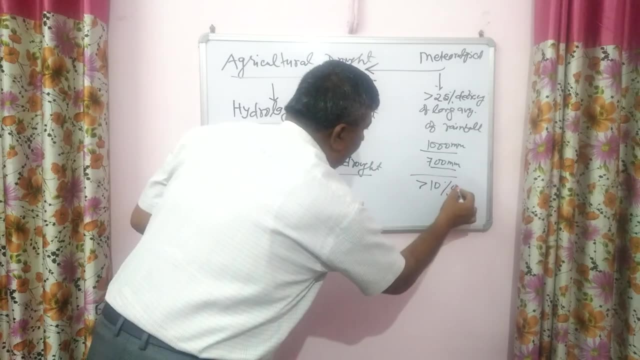 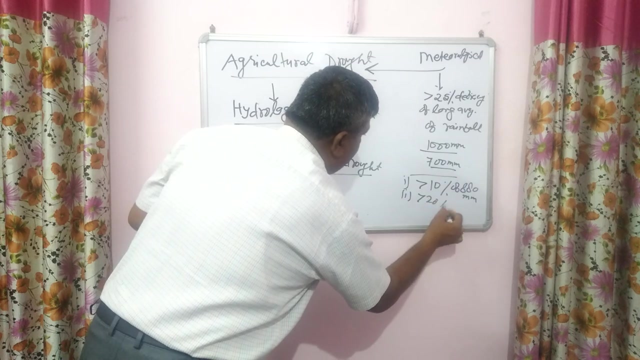 the monsoon is 880 mm. If we want to see the country's metrological dot, then that should be more than 10%. One is there is 80% deficiency of 80 mm in 20% area. pay attention to that. it can be. 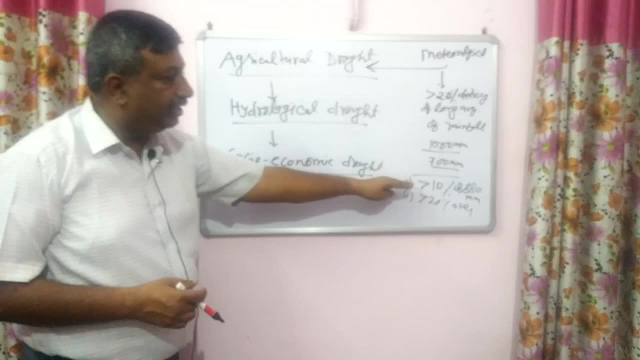 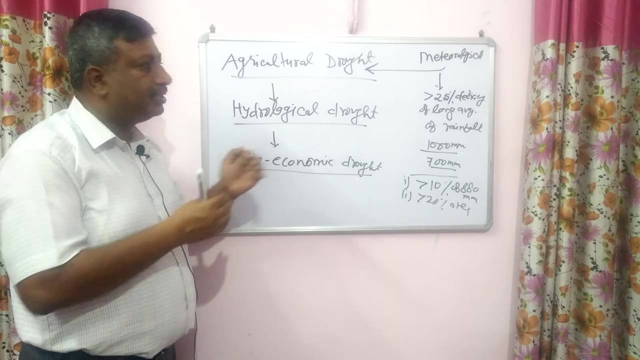 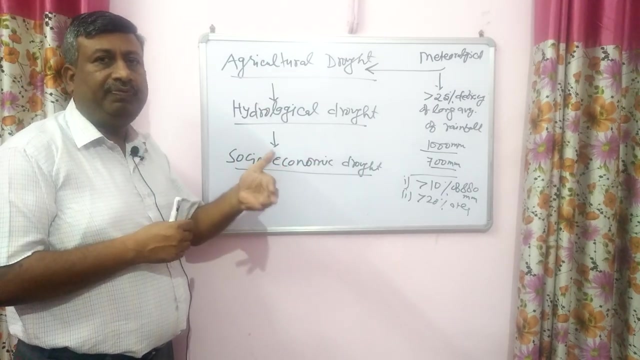 asked in any exam. Second, more than 20% area should have more than 10% deficiency. in more than 20% area there is more than 10% deficiency of this long average. The agricultural drought is when soil moisture is not sufficient to fulfill the plant water. 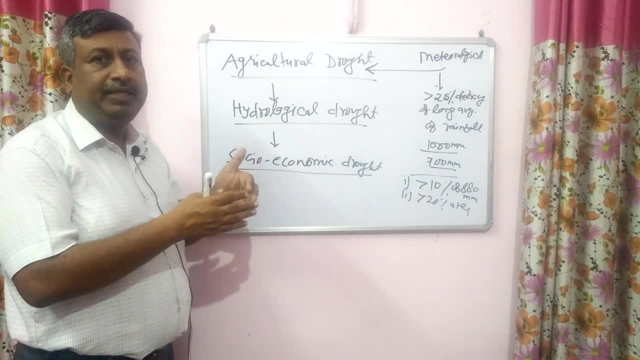 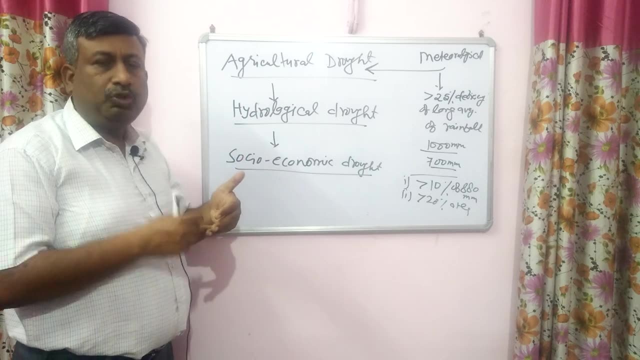 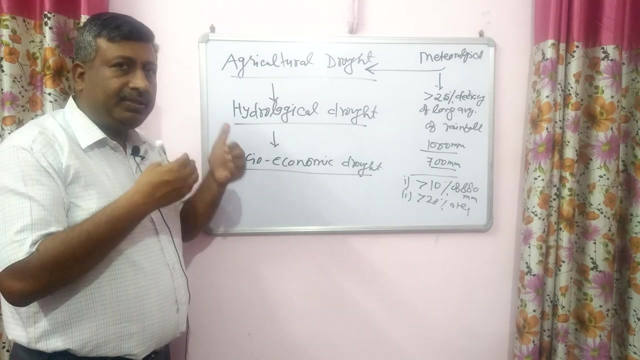 requirement. then agriculture drought and it vary crop to crop. it is relative, it is not fixed, there is no quantification of it. Hydrological drought when in water bodies, whatever the water body is, whether it is a river, a pond, a drain, wherever the water is collected, if the water level is getting. 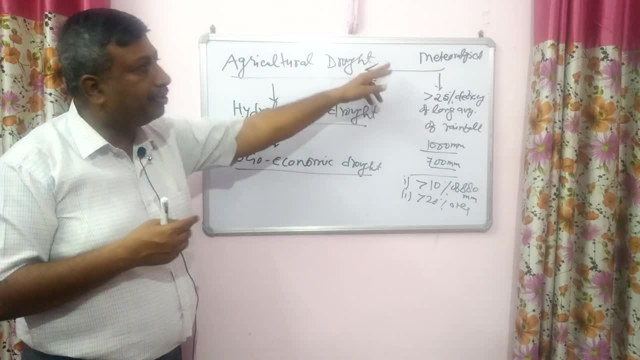 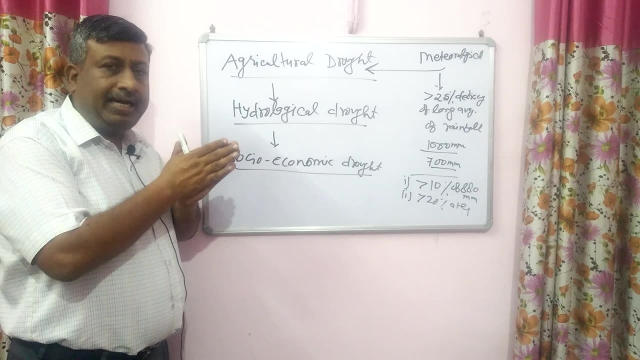 down in the ponds. that is hydrological drought. Why is this happening? Because the rainfall is decreasing And if the water level is getting so low, water availability is so reduced that daily work is affected. human life is affected, industrial work is affected, electricity production. 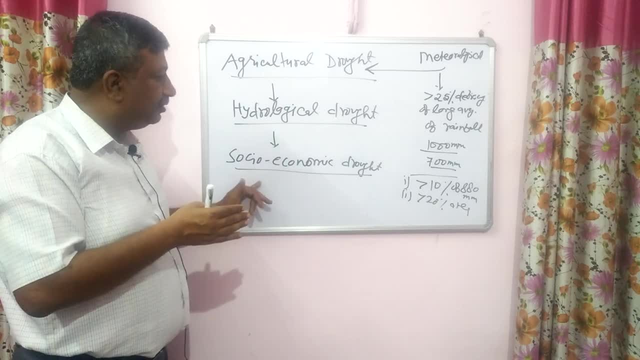 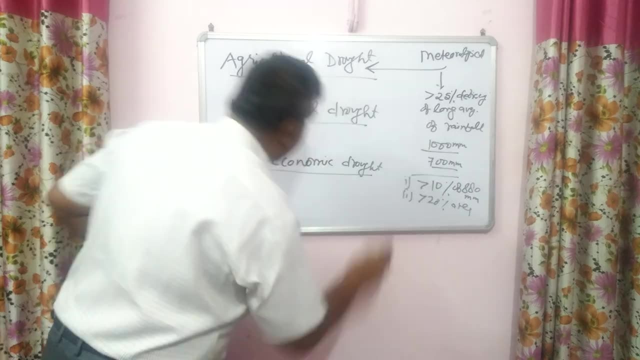 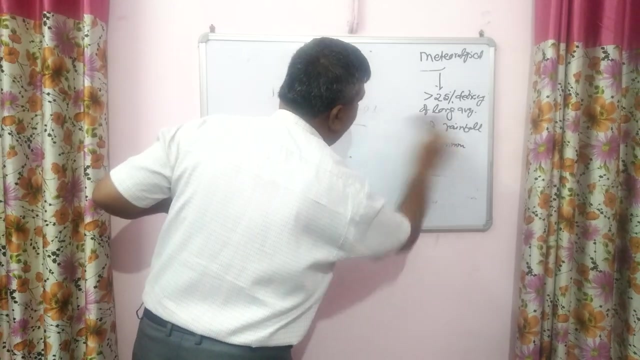 is affected, So all the work related to water is affected. then it is known as socio-economic drought. So there are four types of droughts. these are very important, these four types of droughts, and there are two more droughts which are not in its category, but we should know what. are two different types of droughts: The drought which is not in category and because these droughts are related mainly with monsoon rains, in sequence Then there are other droughts. this is not in four categories. we can call them different. First one is Physiological drought. this is related with the physiology of the plant. 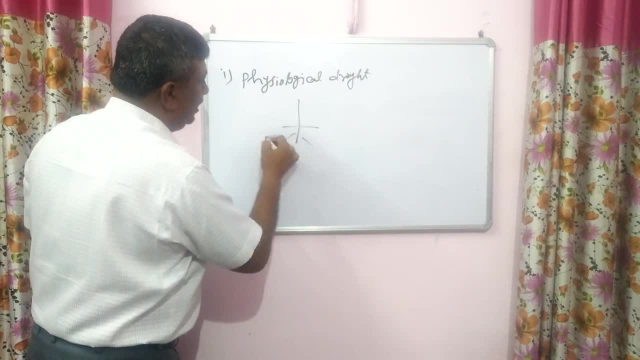 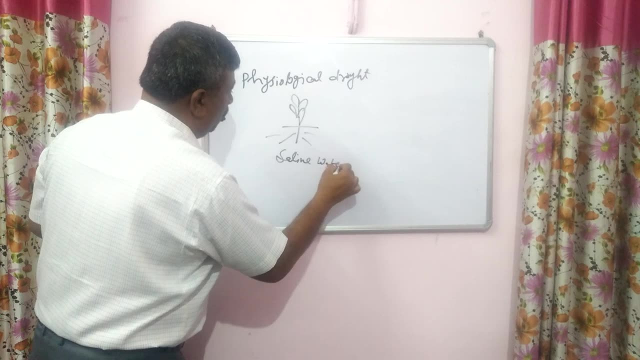 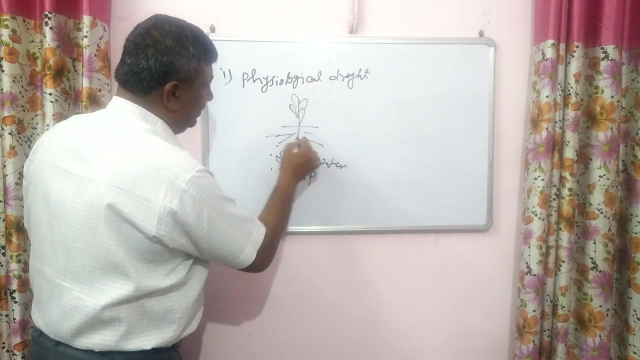 Then this physiological drought is when soil water is saline- This is a plant- and water is saline, then osmotic potential is very negative or very low. osmotic potential is very low. salts are present in it. saline water is present, then roots cannot. 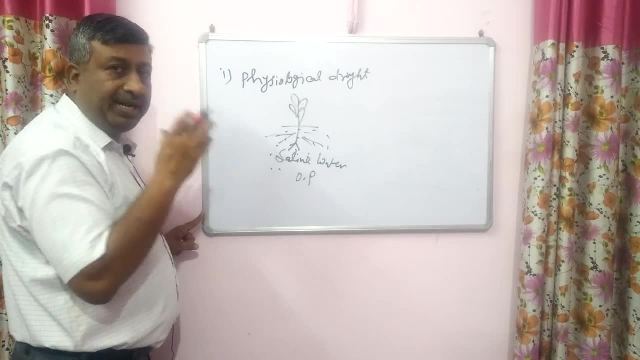 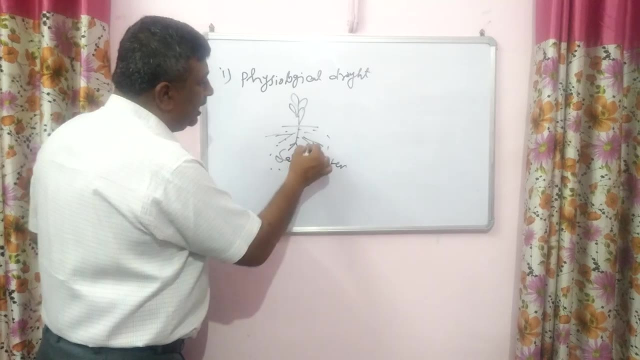 absorb the water. The water is present in soil but because of negative osmotic potential, as much as salt is present, salinity will increase. osmotic potential will be on the negative side. then plant cannot absorb this water and then water deficiency occur in plant. 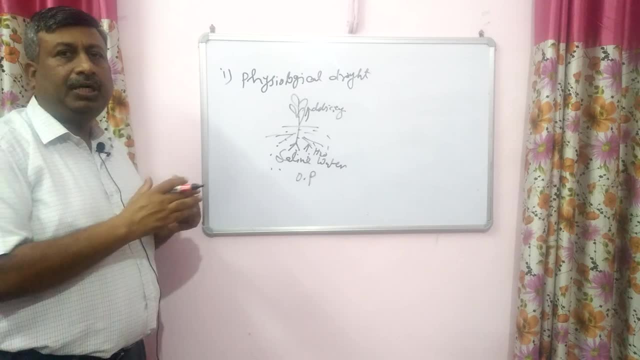 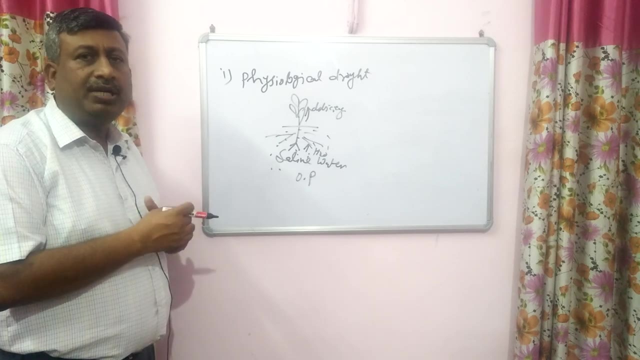 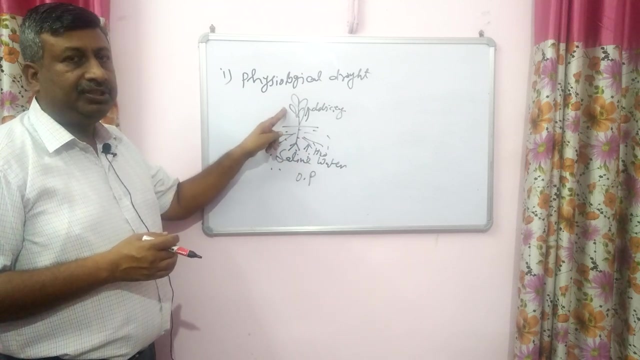 This is known as physiological drought. So in such a condition where salinity is very high, plant root cannot absorb water. saline water plant root very high saline water cannot absorb. Water is present in soil but not available to plant. then there is water deficiency symptom. 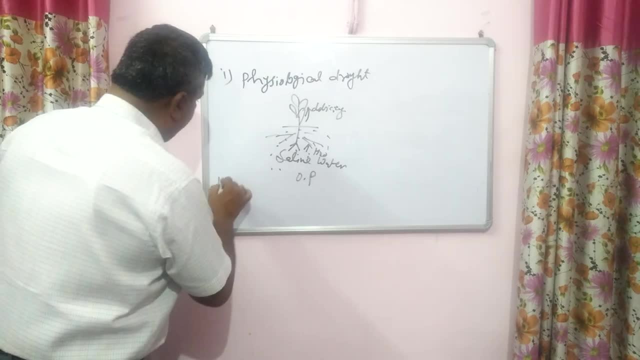 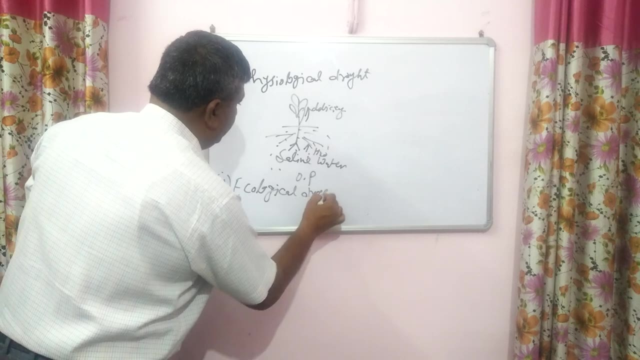 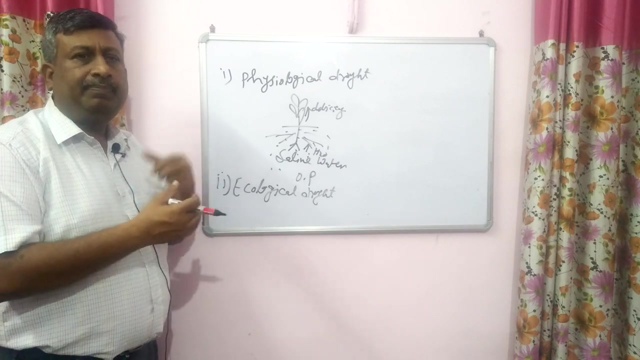 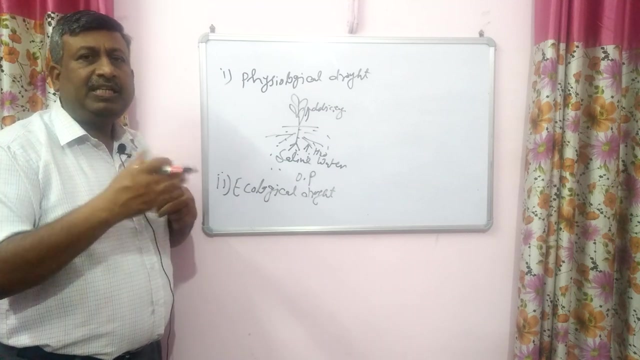 It is known as physiological drought. Second one is ecological drought. In case of ecological drought, there is an ecosystem we know. in ecosystem there is an established ecosystem: forest ecosystem, water ecosystem. there are many species are interrelated. When there is a moisture deficiency or rainfall deficiency, that one species is adversely 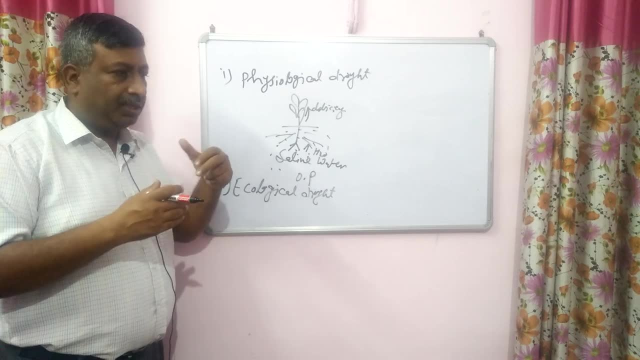 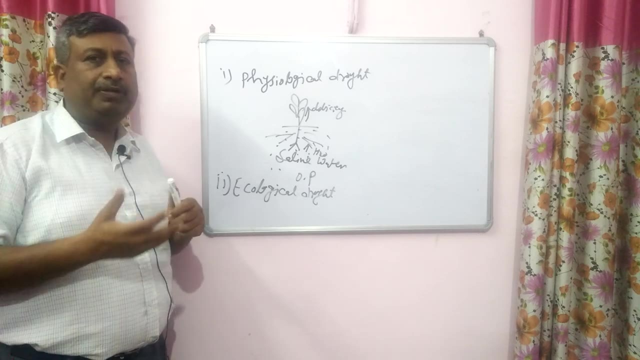 affected, then function of this ecosystem are adversely changed, then it is known as ecological drought. In any ecosystem, any species is adversely affected. In any ecosystem, any species is adversely affected, Any species gets destroyed, Because, you see, in an ecosystem there are many species which are interrelated, which are 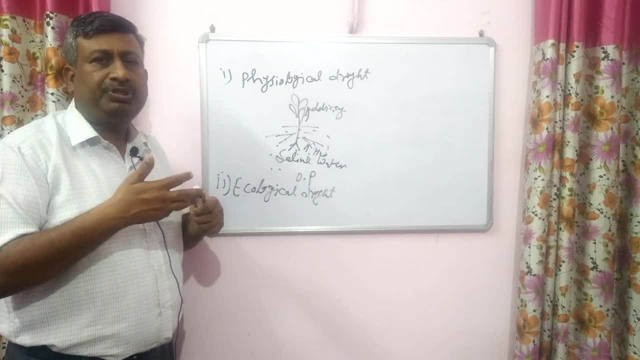 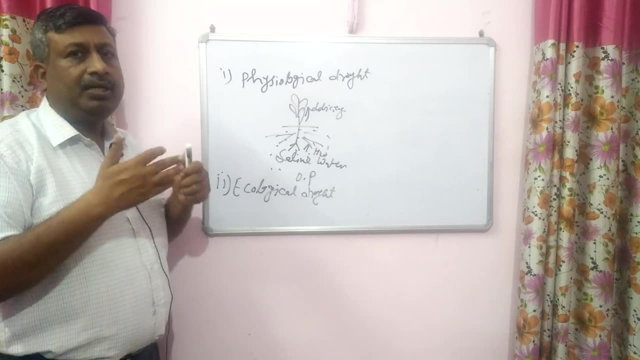 helpful and there are many functions of ecosystem. It is the ecosystem of water, or it is the ecosystem of the forest, or it is the ecosystem of the field. If the rainfall is so less, there is so much moisture deficiency that any species is getting destroyed, then definitely ecosystem is adversely affected. This adverse effect is known as ecological drought. If the rainfall is okay and no species is getting adversely affected, then the ecological drought is normal. then it is not considered as ecological drought. So in case of ecological drought one of the functions of ecosystem are adversely affected. Huge, at huge level. Like there are many ecosystem functions. one function gets adversely affected, one species gets affected, one vegetation gets adversely affected, one animal species or any other species, biota gets destroyed, then ecosystem gets adversely affected. That is known as ecological drought. 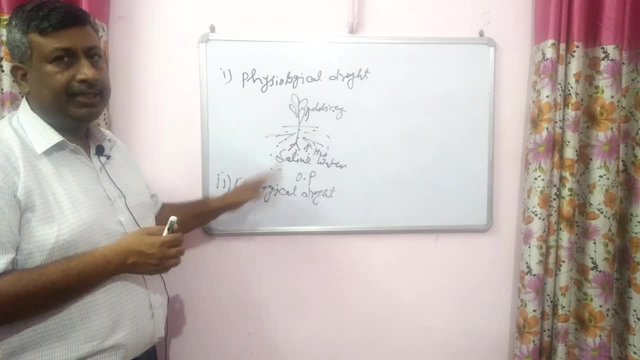 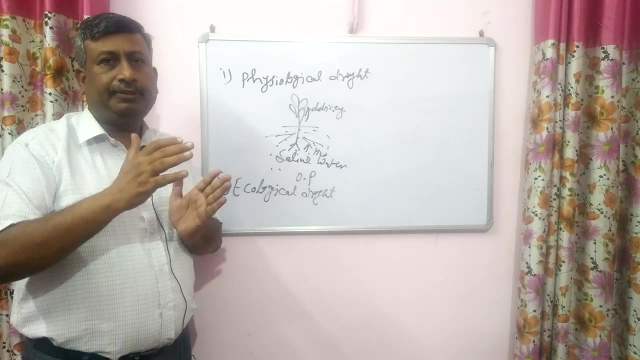 It is related with the ecosystem. So I have told you two different things. Generally, there are four types of drought: Meteorological drought, agricultural drought and last one is hydrological drought and last one is socio-economic drought. So the last important thing is: